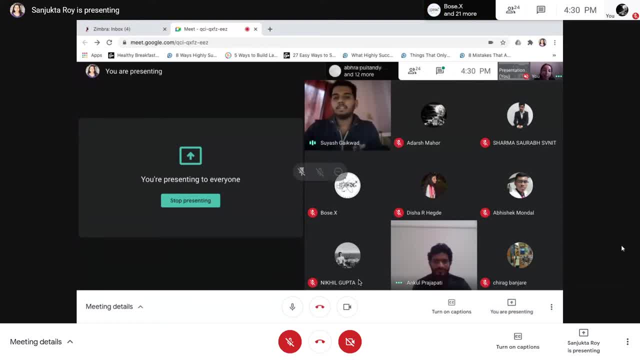 warm evening to everybody. our speaker today is dr sanjukta roy. she is a researcher in atomic physics with a research interest in ultra cold atoms and quantum degenerate gases, with particular interest in fuel body physics with ultra cold atoms and, as she mentioned right now, anderson localization. 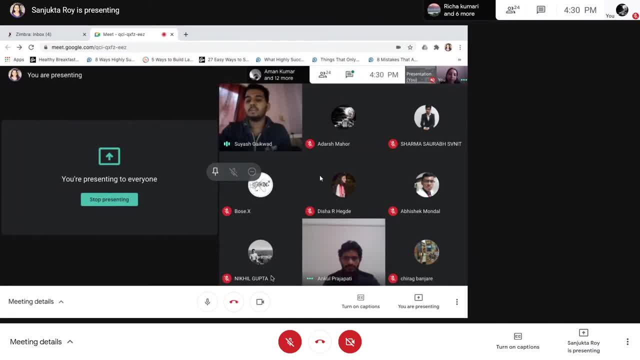 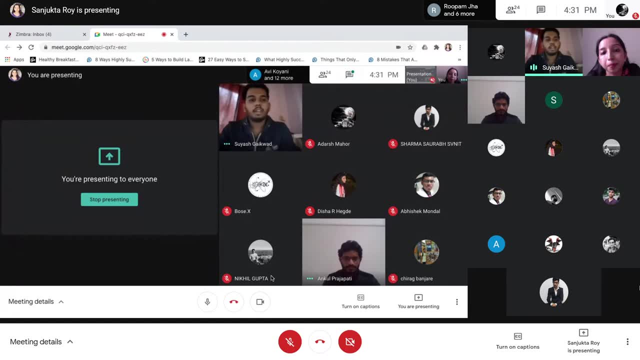 of matter, waves in disorder, potentials and quantum simulations using ultra cold atoms. she is a senior researcher at the raman research institute, bangalore and she did her phd from tata institute of fundamental research, mumbai under krishnan, where she built up an experiment to realize all optical boson condensate in optical traps and 1d optical lattices. the above. 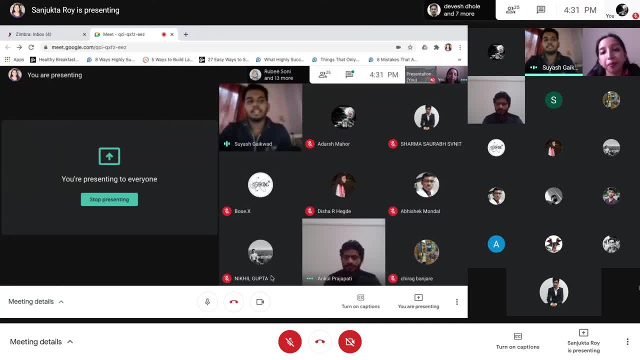 said experiment successfully realized the first bec in india in all optical dipole trap and in 1d optical lattices. she has also worked in uh lkb lab, at ecole normale superior at paris, in the lab of hallam brunette, of Professor Claude Cohen-Tanotji, who is very world famous for his books on quantum mechanics. 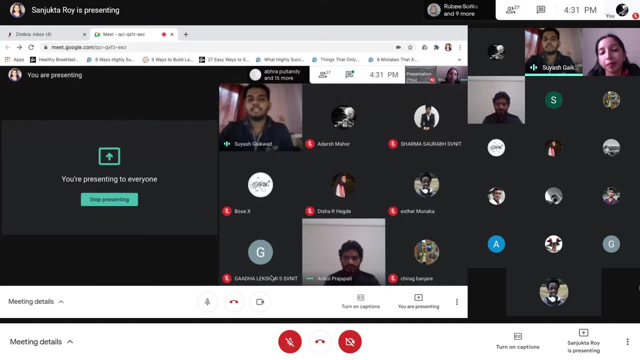 She has a later. she worked in the laboratory Charles Fabry Institute de Optique in France and later in European laboratory for nonlinear spectroscopy, which is in Florence, Italy, And she's currently working in the light and matter physics group at the RRI. 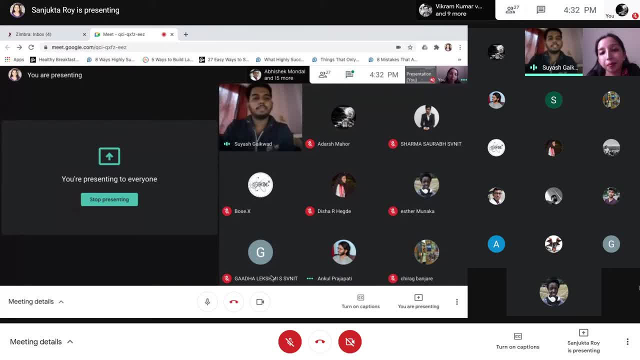 So today she'll be sharing her insights into the field and her expertise in the same, And the instructions to the audiences. I request everybody to kindly switch off their mics till the end, and later the floor will be open for questions. What to use Anjukta. 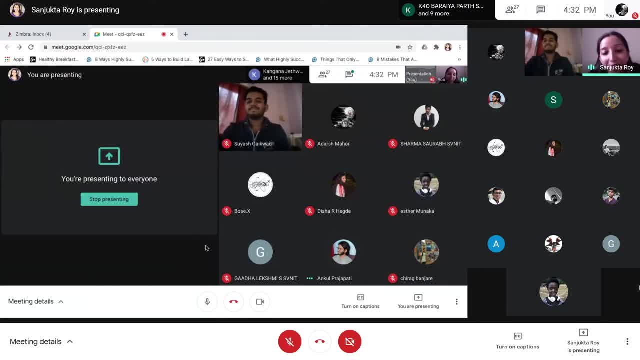 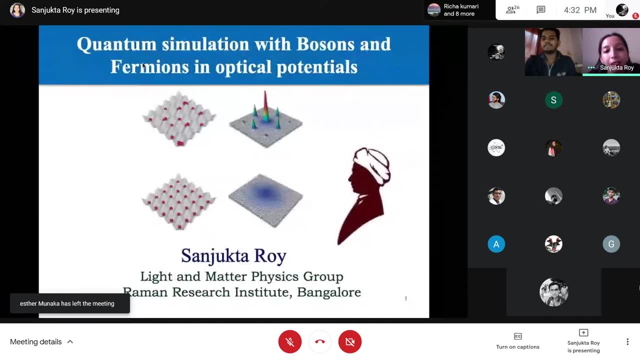 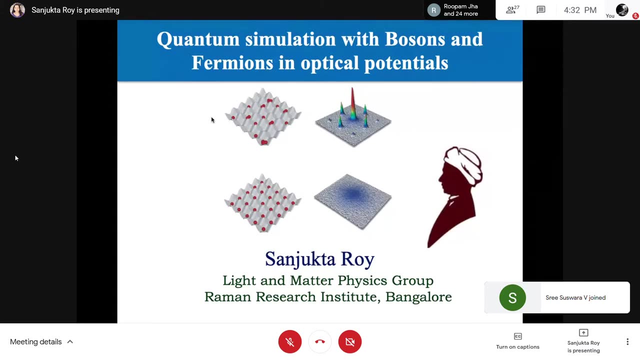 Thanks, Siyash, for the nice introduction. So I start my presentation. So is it visible to everyone? Yes, No, ma'am. Now is my screen visible? Yes, ma'am, Yeah, it is actually visible. The ones who are facing problems may just try pinning. 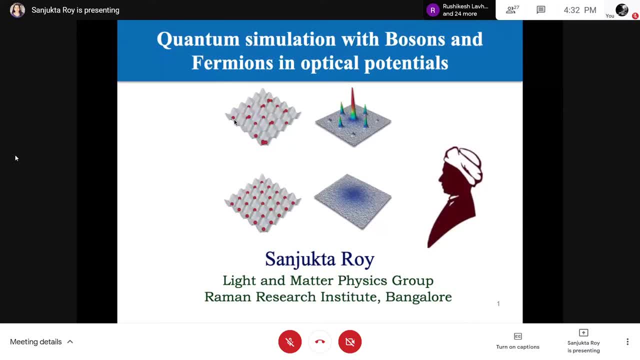 Yes sir, Yes sir, Visible sir, It's visible right. My slide is visible. Yes, ma'am, So I start. So today I'll be talking about actually the main theme of my research, which is quantum simulation. 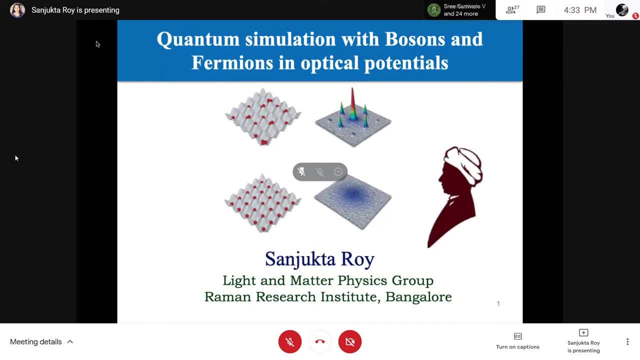 with the bosons and fermions and optical potentials. So I'm as Siyash had said in the introduction, so I have been working in a few labs in India and in Europe And I'm also presently working at the Raman Research Institute. 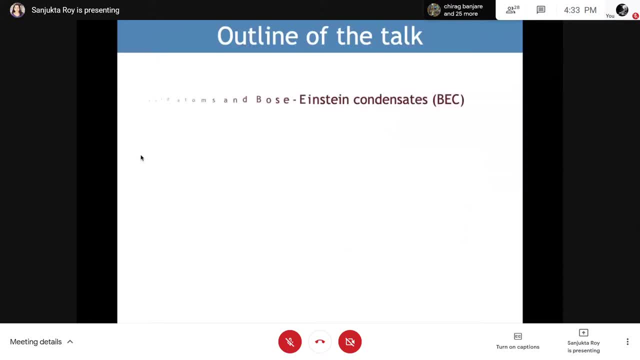 So this talk will be. first I'll give an introduction, Introduction to ultracold atoms and Bose-Einstein condensate. Then I'll actually describe the experimental setup and methods for realization of VEC, Describe optical lattices which are actually. 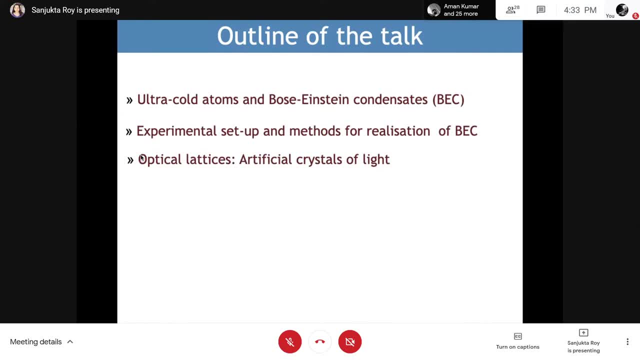 artificial crystals of light, And this enables quantum simulation with the ultracold atoms and VEC in the optical lattice. And then I will show how quantum simulation of open problems and condensed matter physics can be done using quantum mixtures and optical potentials. 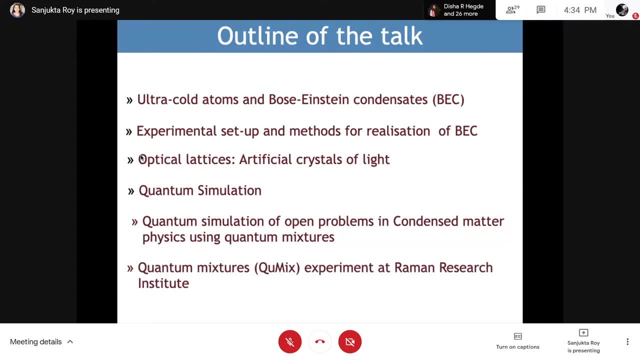 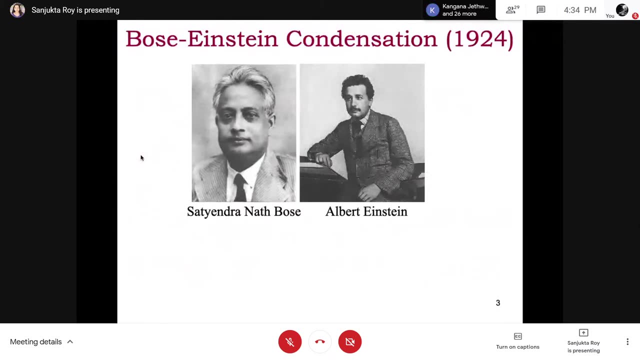 And then I will show a few slides describing the quantum mixtures experiment at Raman Research Institute. No talk about Bose-Einstein condensation can begin without me. I will just do some Motivational analysis so most of you can. you can begin without paying a tribute to the great scientist. 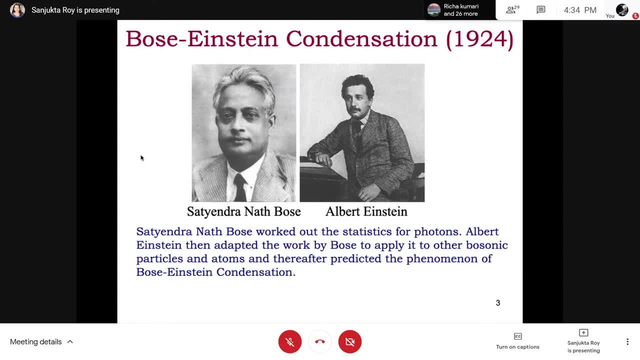 Sethendranath Bose and Albert Einstein. Sethendranath Bose had worked out the statistics for photons, So he was actually teaching and Thaka University and, to answer a question from one of the students, He actually worked out the statistics, which is known as the Bose statistics. 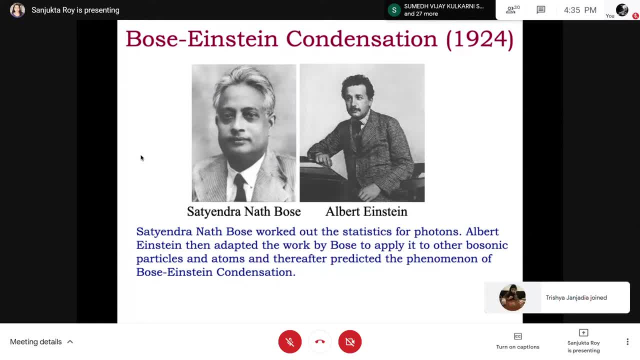 for photons, and then he found the results quite interesting and then he sent his results as a paper to Albert Einstein to to get it published in in a well-known German journal, and Albert Einstein immediately realized the importance of his work and then he adapted the work by Satyendranath Bose. 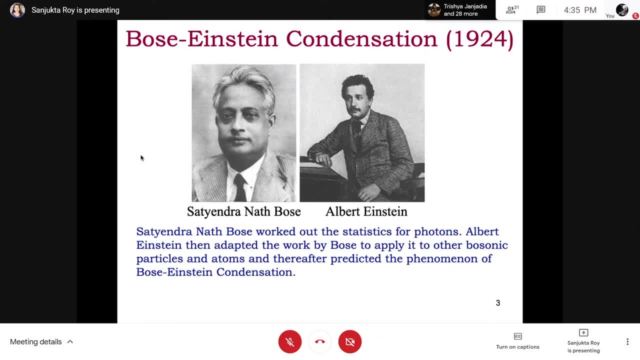 to apply to Bosonic particles and atoms, and thereafter he predicted the phenomena of Bose-Einstein condensation. So it was. Bose-Einstein condensation is an exotic phenomena Which was first realized in a strongly interacting system of superfluid helium in 1938, But it took. 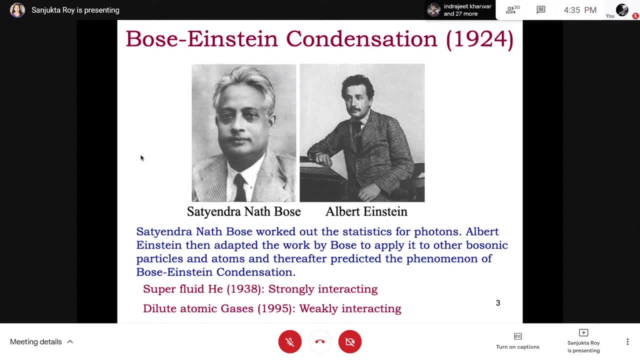 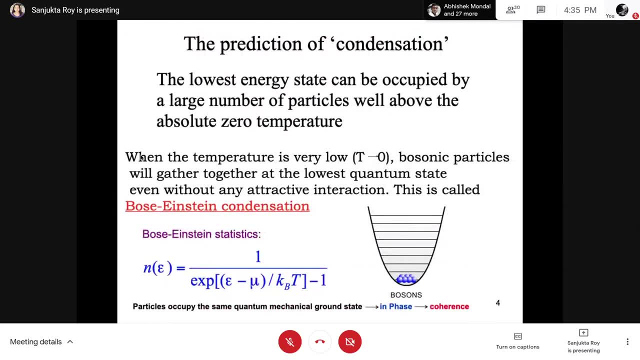 70 years to actually realize in a weakly interacting system of dilute atomic gases. So what is the prediction of condensation? So what is the prediction of condensation? It, the predictions states that the lowest energy state can be occupied by a large number of particles. 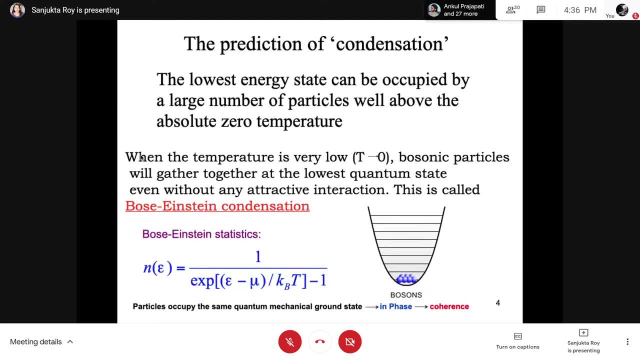 Well above the absolute zero temperature. When the temperature is very low, Very close to absolute zero, Bosonic particles gathered together at the lowest quantum state, even without any attractive interaction, and this phenomenon is called Bose-Einstein condensation and this is, in this phenomena, all the particles. 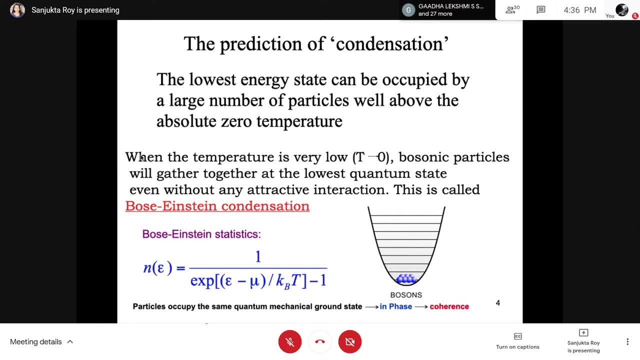 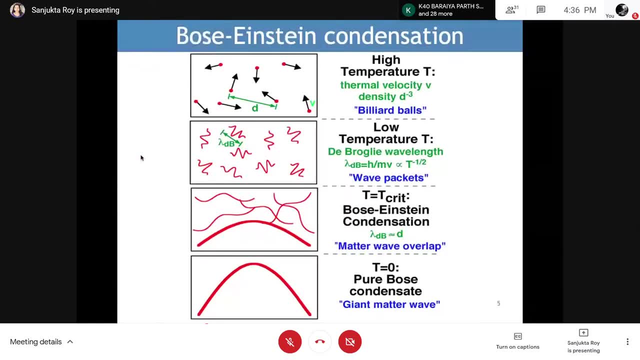 Occupy the same quantum mechanical ground state and they are in phase and that means we can say they are phase coherent. So let me explain Bose-Einstein condensation in in simple terms. so then, at a high temperature the atoms behave like like classical particles, Like like billiard balls. 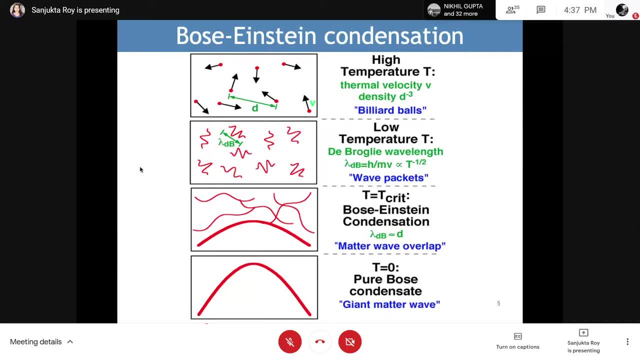 But as the temperature is reduced, So as the temperature is reduced, the de Broglie wavelength of of the particles, which is actually inversely proportional to the square root of temperature, that increases. so as the temperature decreases, the de Broglie wavelength increases. that means 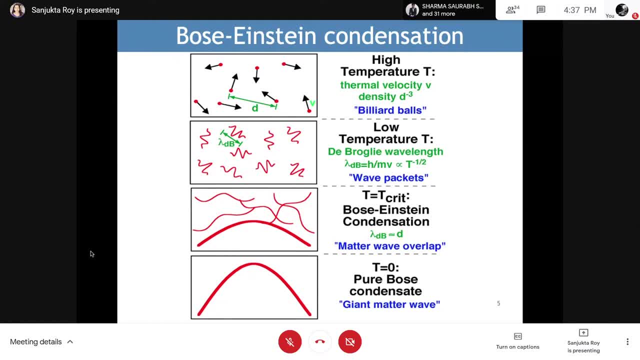 at lower and lower temperatures. the quantum Of the particles are manifested, more and more Temperature. we have the, the De Broglie wavelength of the particles. they are overlapping together and we get the phenomena of Bose-Einstein condensation. Very low temperature, very close to absolute zero. What we get is a pure Bose-Einstein condensate. 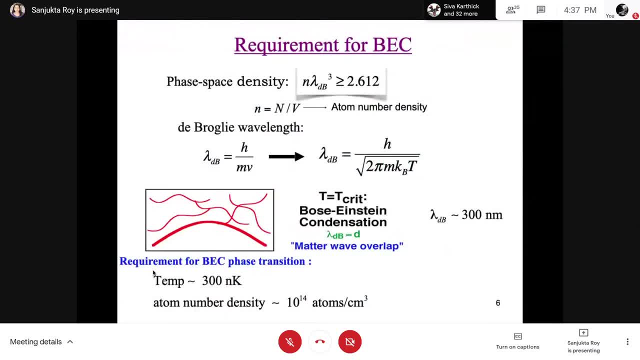 So what is the requirement for a BC? so this is what we experimentalists have to think about when we want to Realize a Bose-Einstein condensate. So to realize a Bose-Einstein condensate, we need to have the phase space density, which is 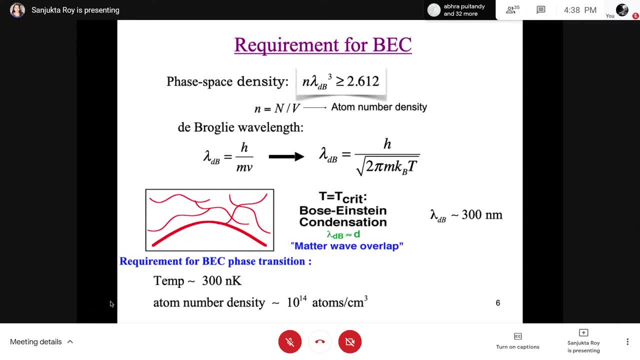 N multiplied by cube of the de Broglie wavelength should be of the order of 1 or are, to be more precise, 2.612. now, n is the atom number, density, and lambda, as I had explained, is the de Broglie wavelength, which you see is inversely. 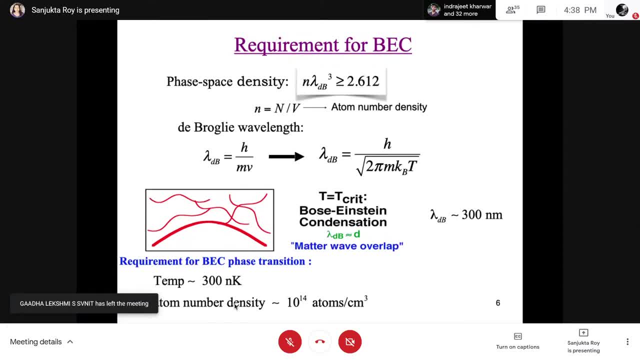 proportional to the square root of temperature. Temperature is reduced to lower and lower temperatures, the de Broglie wavelength increases and at the critical temperature for the BC phase transition they overlap and The the particles go into the Bose-Einstein condensate phase, now at the BC critical temperature. 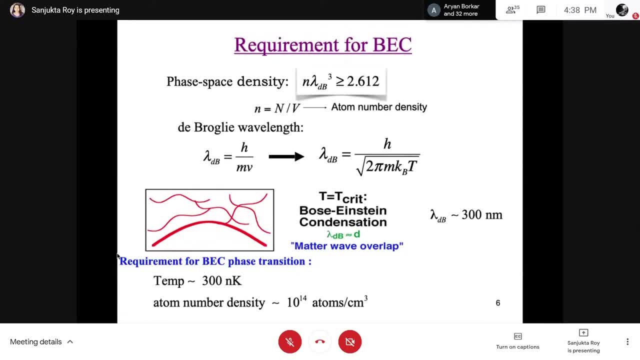 The typical de Broglie wavelength is around 300 nanometer. Now the requirement for the BC transition in terms of temperature and atom number density is like the typical temperatures for BC phase transition is like 300 nano Kelvin and the atom number density is like 10 to the power, 14 atoms per centimeter. 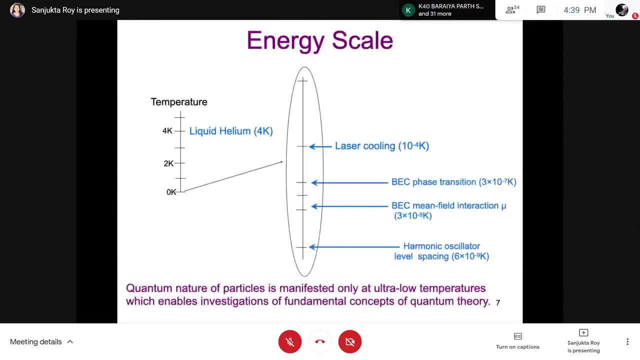 now Let's see where this temperature stands in. you know, you know the temperature scale. So, as we know, liquid helium, which is already very, very cold, the liquid helium temperature is like 4 Kelvin, and Then we go all the way to and if you zoom there, we see that. 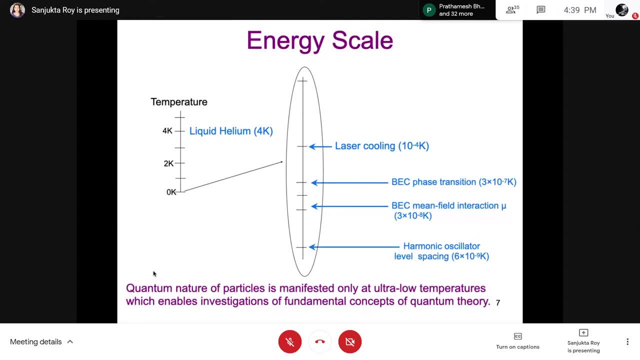 at near zero Kelvin. we have The laser cooling. the temperature for ultra cold atoms is like hundred micro Kelvin and the BC transition temperature is like 300 nano Kelvin. another Advantage of going to very low temperature, as I'd explained that the quantum nature of particles is manifested at at ultra low temperatures. 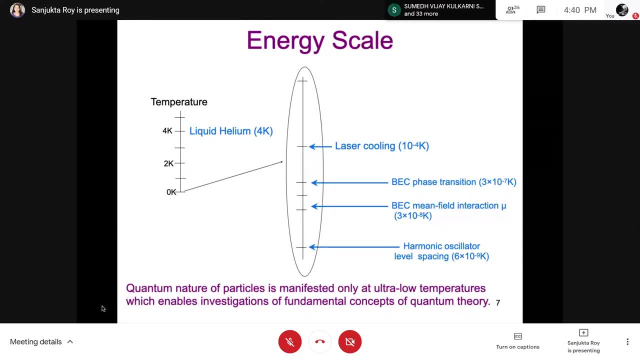 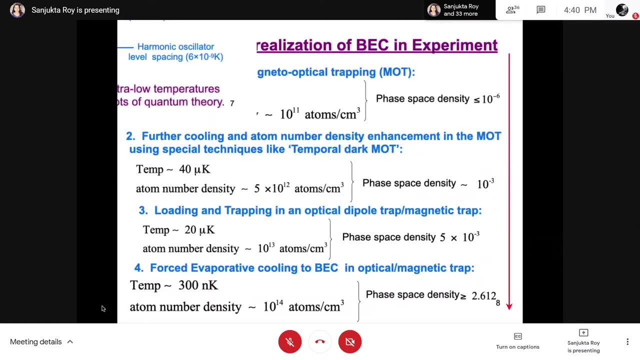 and this enables Investigation- are exploring the fundamental concepts of quantum theory. i Mean, if I would also you know, if you have any questions or need any clarifications. I mean you can without hesitation ask me, because if I'm going too fast you can always ask me for clarification. 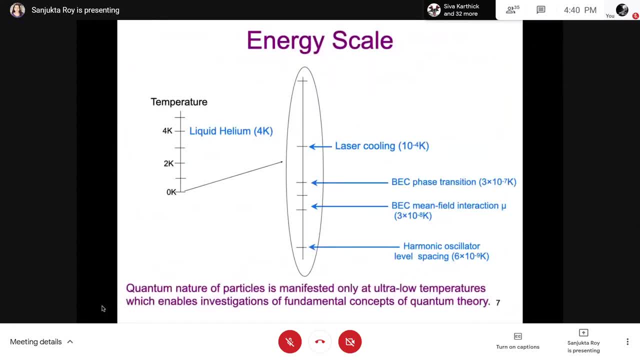 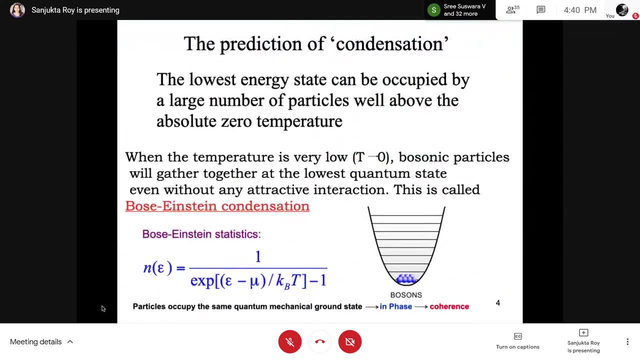 Man. there is the one exercise either can x-ray the home n photon? Yeah, Holiday will begin with each. there's the half spin particle, the fully spin particle. what is the visualization of the photon that is the fullest? yeah, it has. it has an integer spin particle. so all the particles which are like uh, for example, we 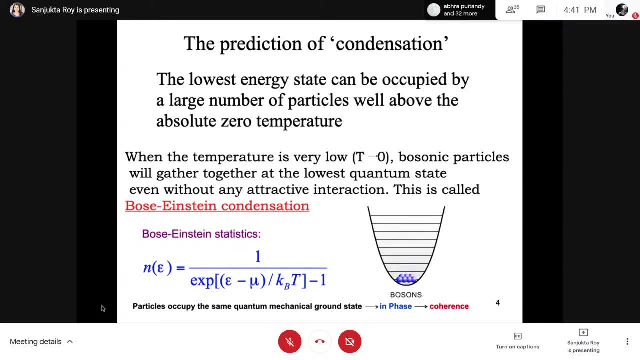 work with ruby etm. it has integer spin particle and the particles which have like half integer spin, which are electrons or you know um. so there are many other other particles which are like half spin, uh, for example, in in elements also, you, you uh actually have bosons, depending on what is. 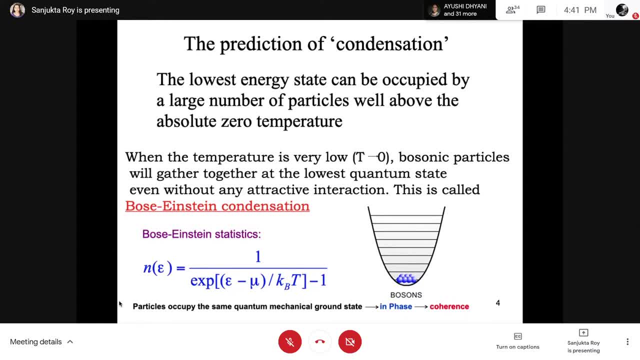 the total number of the nucleons. okay, so what is the total spin of the atom? so if the total spin of the atom is integer- you have you call it a bosonic particle. or if the total spin is, uh, is half integer, you have call it a harmonic particle. here is right as the absolute temperature above. 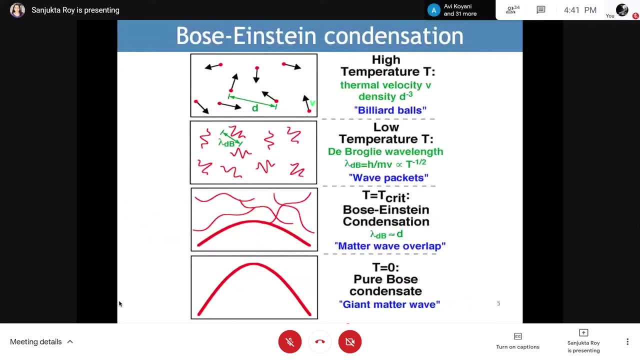 the is it possible to acquire the absolute zero temperature in case of the? uh? no, it's not, because it's against the uh, i mean it's, you know, it's a. the theorist can actually do the calculation using uh, absolute zero temperature. but uh, it's, uh, it's not. uh, you know, in experimentally or in practically, it's not. 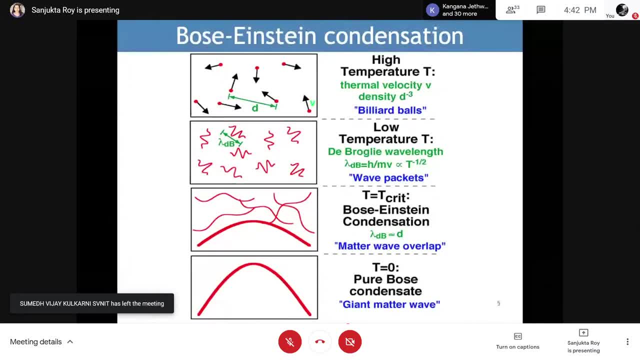 it's not possible. but we can go very, very close to absolute zero temperature and the lowest one has gone, uh is it's in mit um, in the group of wolfgang cattley. they have gone to around a few hundred pickel kelevins of temperature, so that's the lowest record temperature to now. 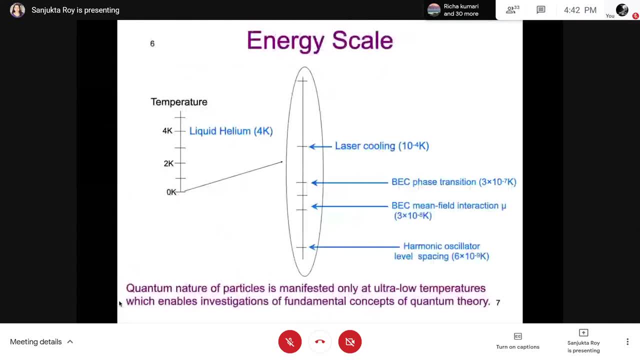 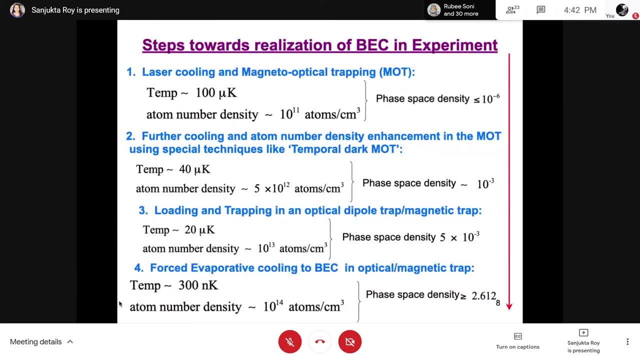 ok man thank you so the step towards realizing a Bose-Einstein condensate is quite involved and it involves several steps uh so i won't go into too much details of each of the ev��라고요Sam萬자 나�abe 150 verдж 기간 � etap은 몇PO 메리ties 자 전체 한 가지, uh, so i won't go into too much details of each of those. we're going to Ando자 the很. 일단, 정Q join me in considering basalt 원화 Income to ando demande. 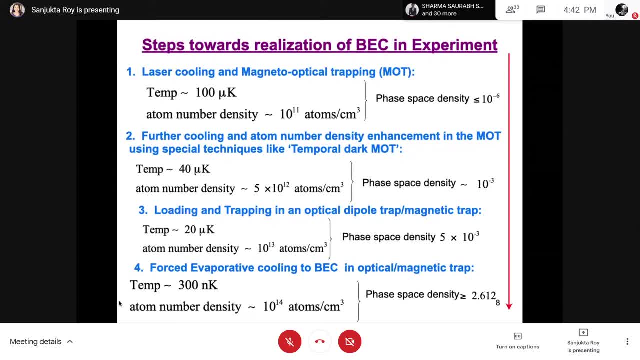 uma e vanilla process. all these factors are greatly different. so in between, for example, in which you can take the Lösa you чер' fo' 바�生hand' the step, but i would like to, you know, highlight the main points. so what are the, uh, the steps? so 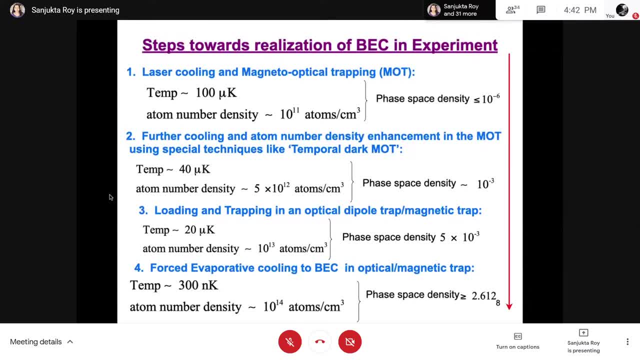 first and the foremost important step is laser cooling and magnet optical trapping. uh, so there, you can actually lower the temperature from the room temperature to around 100 micro kelvin temperature and get a atom number density of around 10 to 11 atoms per centimeter cube. and 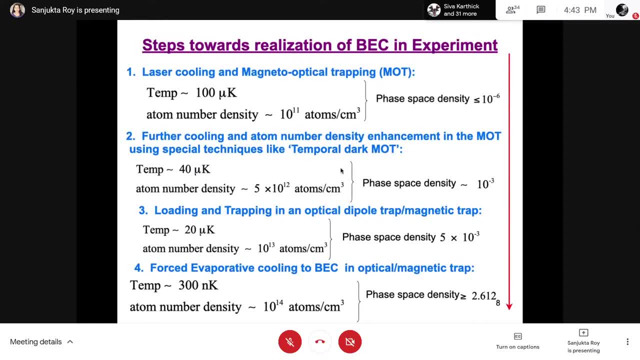 uh, still here. the phase space density is 10 to the power minus six, way less than the phase space density required for the bc, which is like of the order of one. so there are several steps, as you can see, to get the bc. so the first is the laser cooling and trapping, which actually cools the 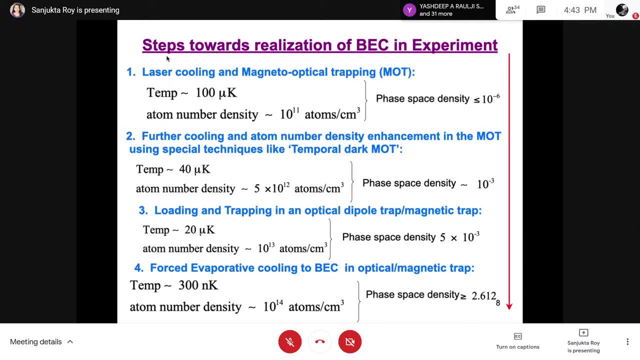 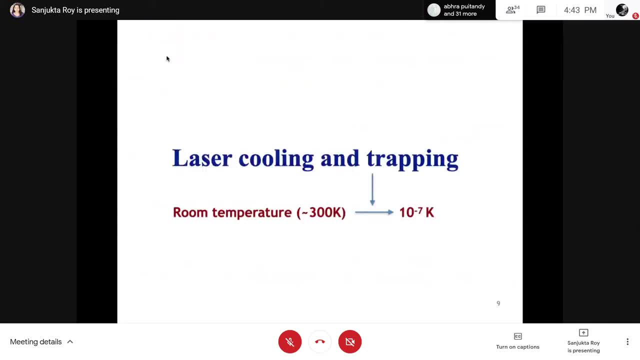 atoms from the room temperature right uh all the way down to around half kelvin temperatures. so let me explain what it is. so, as you can see, that laser cooling uh reduces the temperature from around room temperature of 300 kelvin to around 100 micro kelvin temperature. now how does it happen? so generally we think about 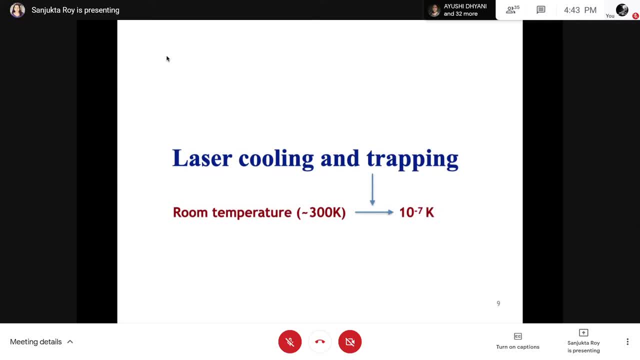 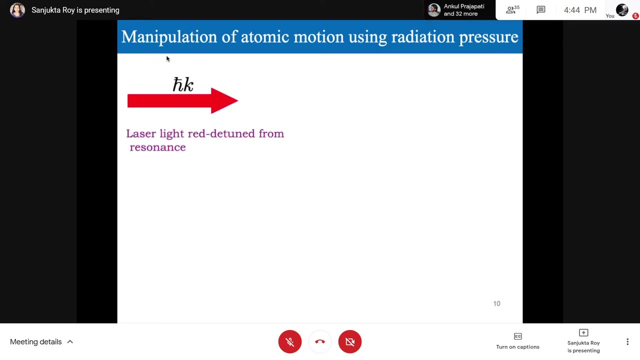 uh, you know lasers as heating up things. so how does it actually cool the atoms? so, uh, let's see, how do we manipulate the atomic motion using the radiation pressure from the laser beams. suppose you have a laser beam which is uh moving um towards, uh in the opposite direction, uh as the atom. so if that uh, 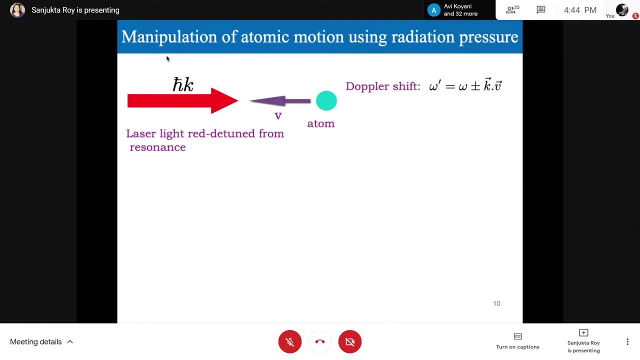 laser beam with the velocity b, v and because of the doppler shift, the atom actually sees the frequency of the laser upshifted. now, if you see, this is the- uh, you know- ground state in the excited state and if the transition frequency is like omega, so if the laser is already um ready tuned, that means having a frequency. 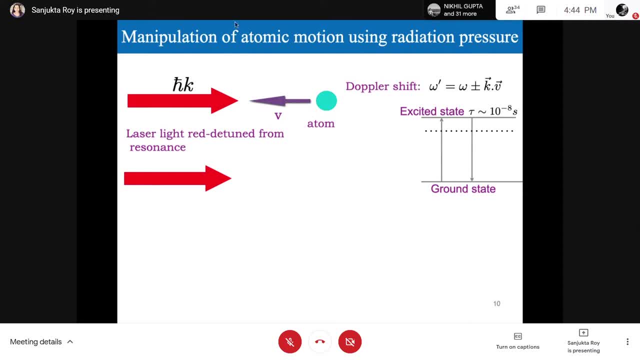 less than that required for that big transition. so, uh, the atom will see the laser beam upshifted because, uh, upshift, upshifted because of the doppler shift, and it will find it on resonance. and then the atom will absorb a photon and get a momentum kick opposite to its direction of motion. 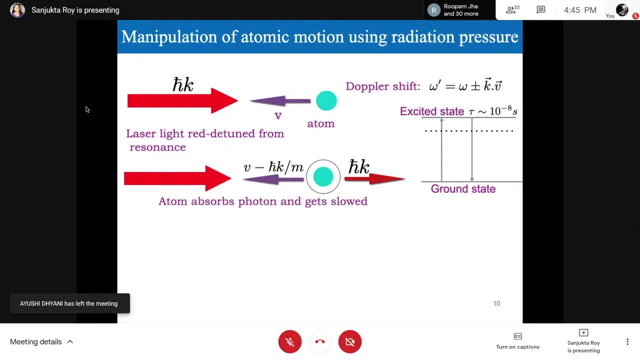 so, as it gets a momentum kick opposite this direction of motion. ma'am, please explain the absorption of the photon by the laser beam. once again, yes, so, uh. so if you assume as a two-level system it's having a ground state and excited state, right now we know that if the laser beam has a photon, 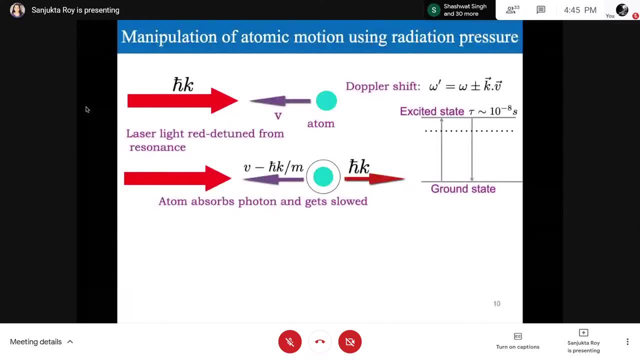 with an energy equal to the difference between the ground state and the excited state, then the photon will be absorbed by the atom. right, yes, ma'am, yeah, so, uh, now we have to take care of the motion of the atom, because of which there is a doppler shift. so there's a doppler. 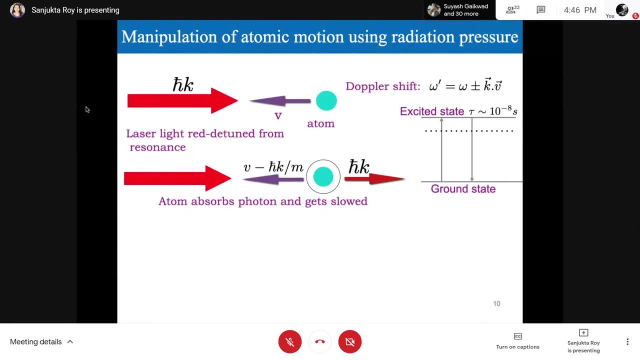 shift. so that's why we already have the frequency of the laser little bit less than the atomic transition frequency. now, because of the doppler shift, the uh atom sees the frequency of the laser beam upshifted and then thereby sees it on resonance and hence absorb a photon from the laser beam. and as soon as the atom absorbs the photon from the 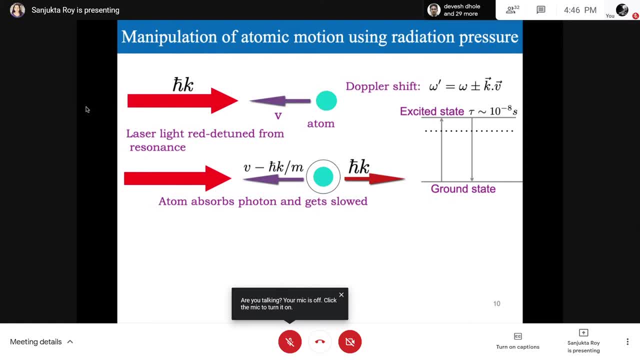 laser beam, it uh, it gets a momentum. momentum kick opposite to its direction of motion and hence gets slowed down. now, as soon as it absorbs the photon, it also emits the photon using spontaneous emission. but that spontaneous emission happens in random direction. so, as you know, in one second they're. 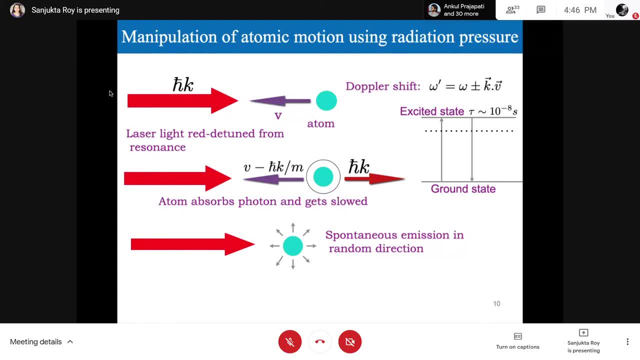 around 10 to the power. six times the atoms absorb and re-emit uh the photon. so at each, each uh, each absorption it gets slowed down. but for the spontaneous emission it happens in random direction. so on an average the effect of the spontaneous emission averages out to be zero. so 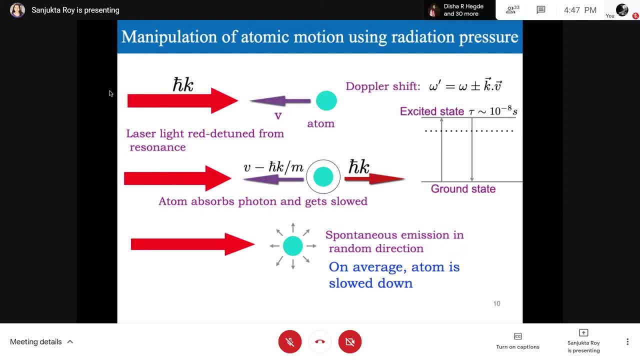 that's what we're going to talk about in a little bit more detail, in a little bit more detail. so what we're going to talk about in a little bit more detail, in a little bit more detail, is the slowdown of the atoms. so the slowdown of the atoms remains is the slowing down of the atom. 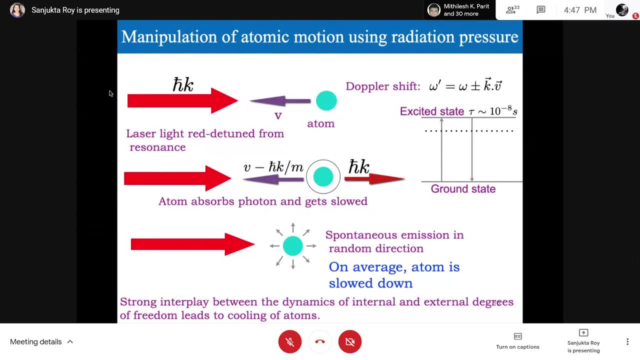 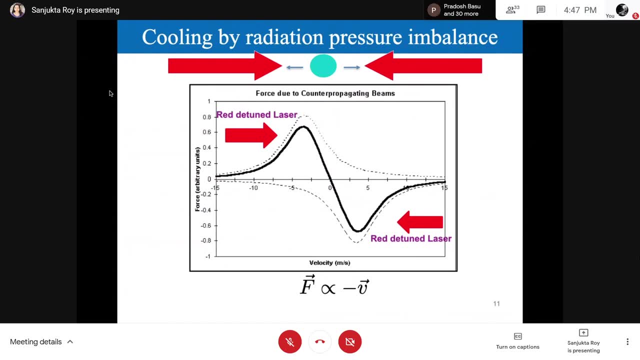 at each of the absorption of the photon by the atom, see that there's a strong interplay between the dynamics of the internal and the external degrees of freedom, which leads to the cooling of atoms. so what happens now if you have laser beams shining on the atoms from both the direction? 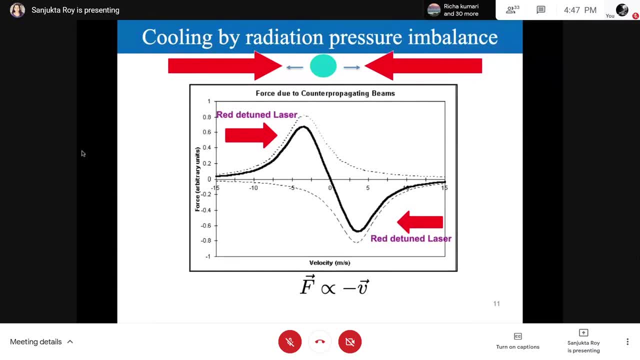 of the laser beam and the direction of the laser beam. from both the direction of the laser beam and the direction of the laser beam, as you can see in this figure, the the force is actually having an opposite sign to the velocity. so that means the force of the laser beam is always opposing. 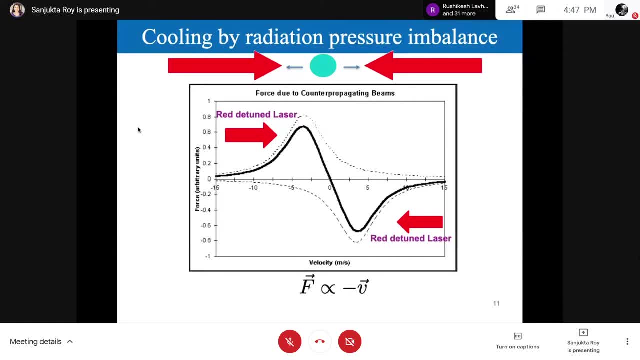 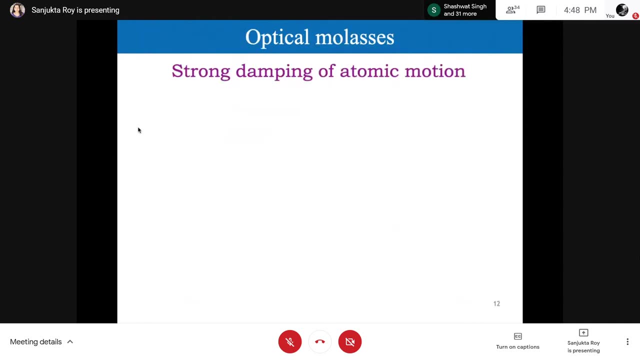 the motion of the atom. so towards the center, at the, the low velocity class, you can see that the force is actually linear proportional to linearly proportional to the velocity. that means it's like actually slowing down the atoms. so if you have the laser beams and all the three, 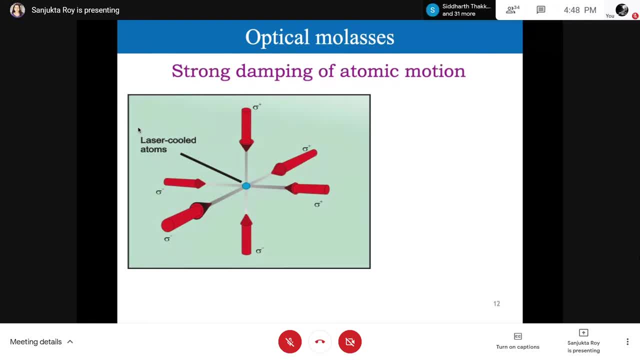 direction, that's y and z direction. what you form is a 3d optical molasses. so whichever direction in in all the three dimensions the atom tries to move, it gets slowed down because of the doppler cooling, by the laser beams, because the atom feels a viscous force. 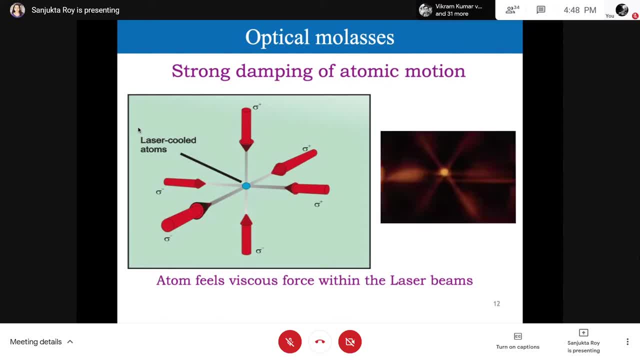 in the laser beams. now here you can see a real picture of of sodium atoms in an optical molasses, so you can see the cold atoms at the center which are cooled down because of ma'am. when the laser beam, when the laser beam will strike to the photon, then the energy will be increased, increases, or 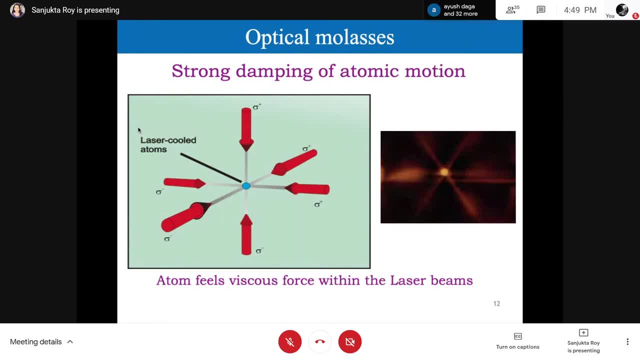 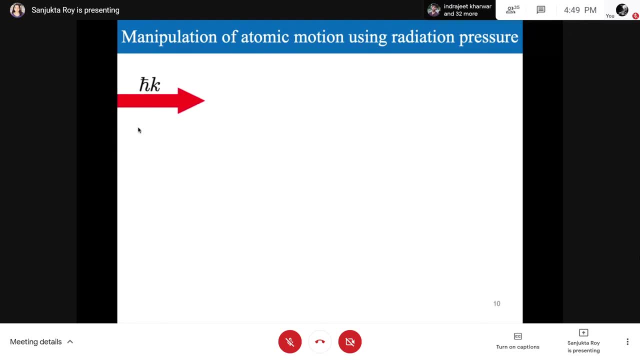 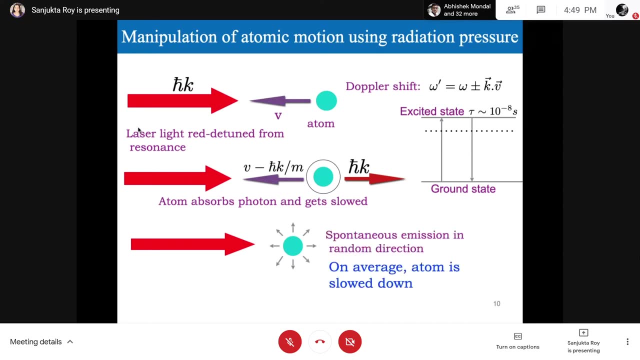 decreases all right of the photon. that's what i have explained till now that uh see in the earlier slide. so it is actually uh also following the conservation of energy. see, the atom is on at lower energy but when it's doing spontaneous emission it's actually emitting. 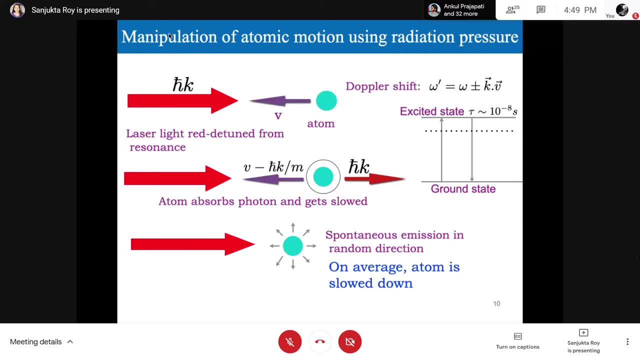 at higher energy. so this difference in energy is actually dissipated and taken away by the photon. is it clear? so that is actually taken. this extra energy is taken away from the photon and it's going away from the kinetic energy of the atom and thus the atom is getting slowed down. 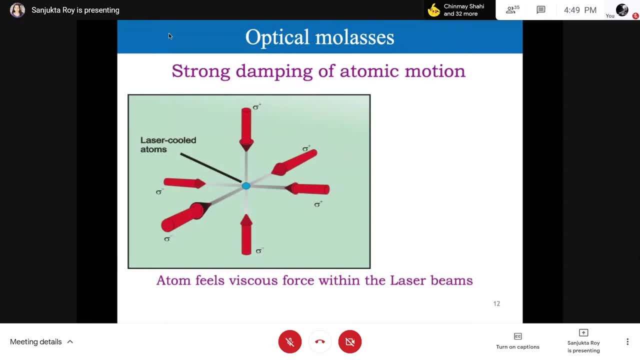 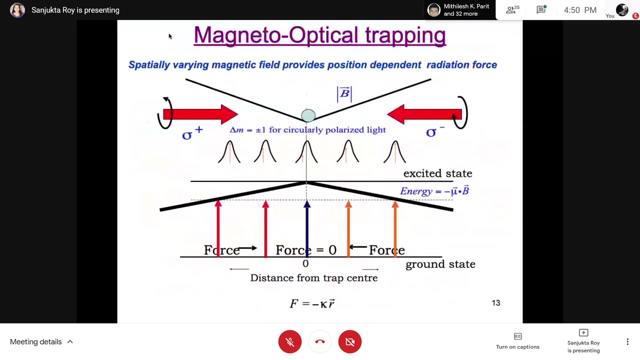 yes, ma'am, yes, ma'am. so, uh, but this is only damping for us, so there is no trapping at a point in space. so how do we do the trapping? we use something called a magneto optical trapping. so for this we use a spatially varying magnetic field. 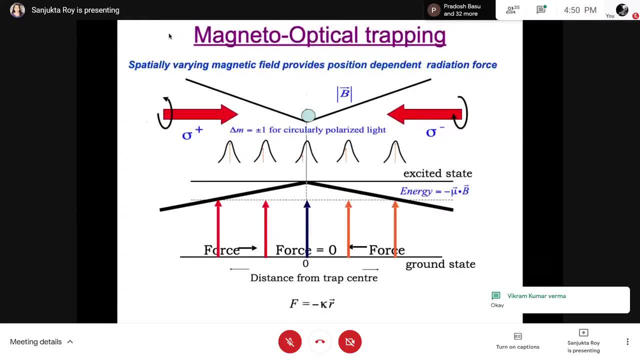 which is actually zero at the center and, uh, it's increasing linearly in all direction. let's slide how we actually experimentally prepare it. but now i'm just explaining the concept. now, when the magnetic field is zero at the center and increasing linearly in all direction, so when the 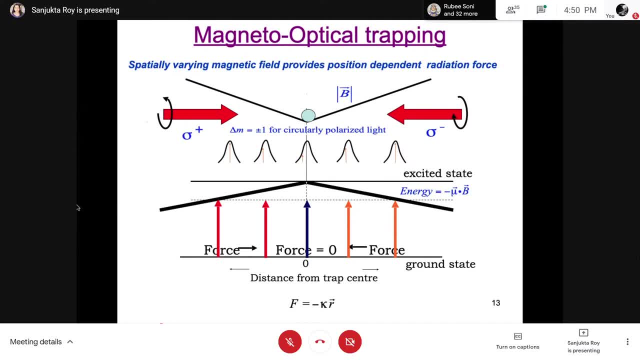 atom is at the center, which is like, uh, really, where we want the atom to be. it doesn't experience any force. but as the atom goes away from the center, it's since the laser beam is already ready tuned. that means having low, frequent, lower frequency than the transition frequency. it comes more on. 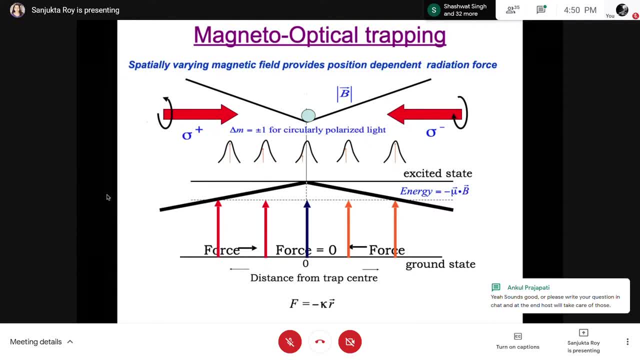 resonance due to the z-man effect as the atom goes away from the center. so the more the atom goes away from the center, more the force it feels, which pushes the atom towards the center. so as it goes away from it absorbs a sigma plus photon, and if it goes to the left side it will absorb a sigma plus. 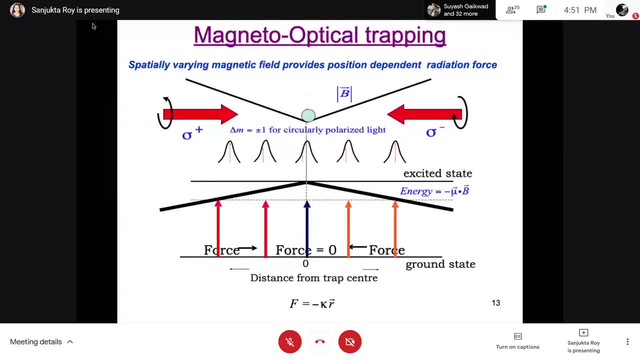 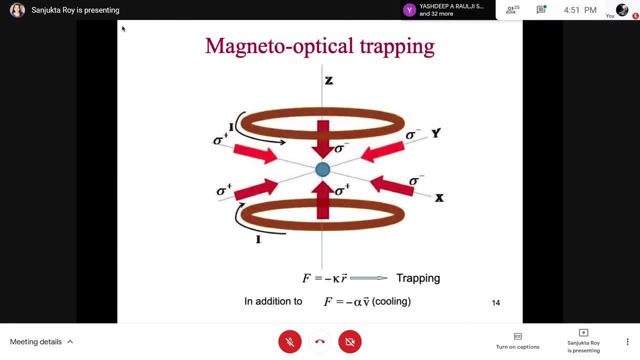 photon and get a force, which is which will push it towards the center, and the same will happen in the other direction as well. so it's like us restoring spring force, which is actually pushing the atoms towards the center. so how do we actually realize it? we use a pair of magnetic coils in what is 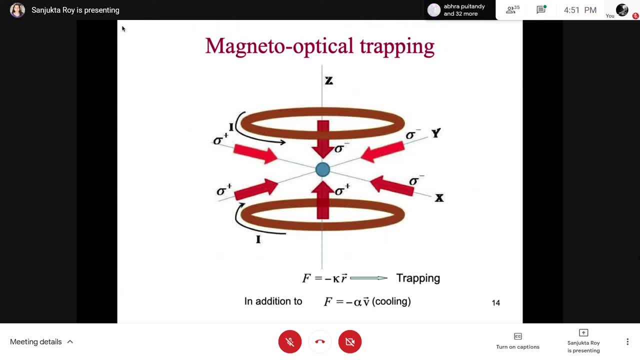 called a anti-hell bonds configuration, with the current flowing in the opposite direction. so this will. this is actually creating a zero at the center and uh, uh and uh and it will create a gradient. so it will increase linearly in all direction, but give you the zero at the center. 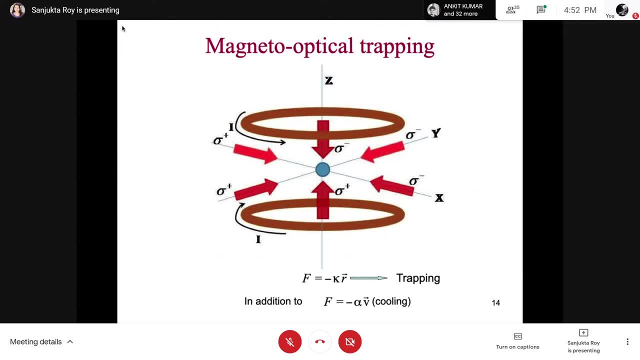 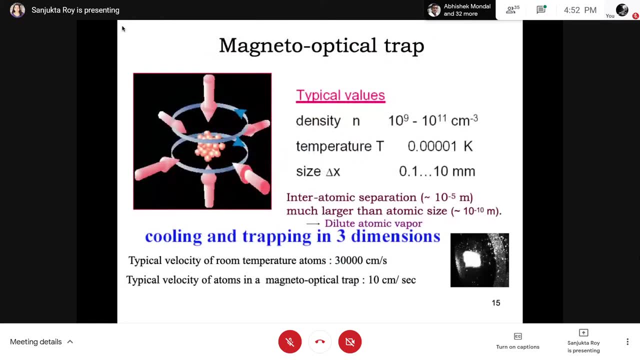 so this is how we can trap, cool the atoms using magnet optical trapping. so, uh, let us look at the typical parameters. in a magnet optical trap, the density is around 10 to the power, 9 to 10 to the power, 11 atoms per centimeter cube. 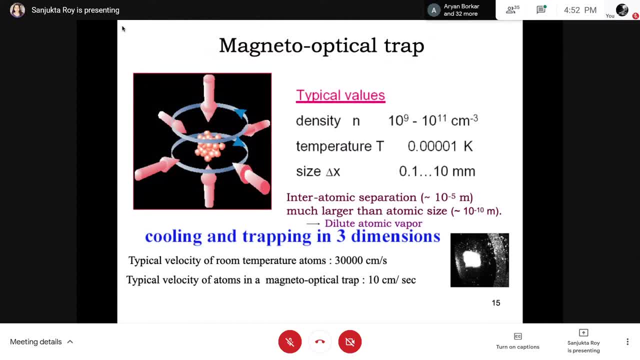 the temperatures is around 100 micro kelvin and we can have a size of the atomic cloud around even from starting from 100 micron to around 10 millimeter. now here, one point to note is that it's still the interatomic separation is like around 10 to the power. 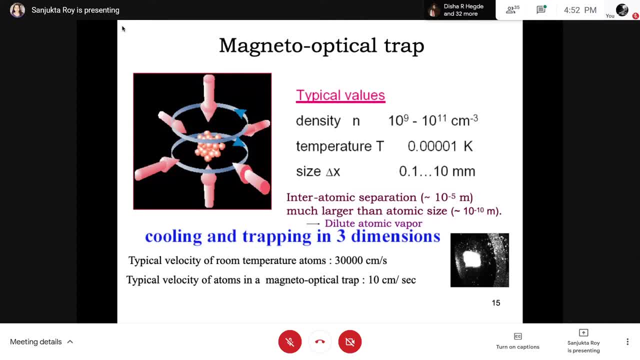 minus 5 meter, which is much, much larger than the atomic size. so this is this. that's why it's a weakly interacting, dilute atomic vapor. now, uh, just to compare the velocity, a typical, the typical velocity of room temperature atoms is like 30 000 centimeter per second. now, compared as compared to 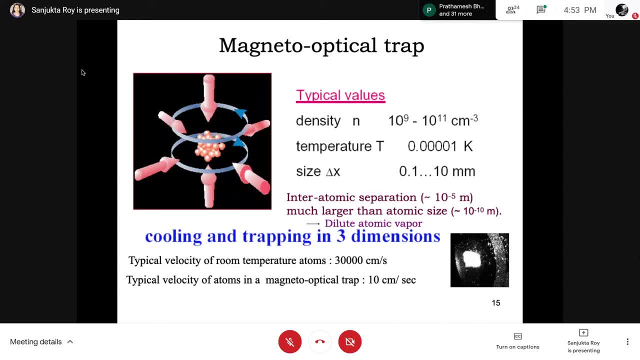 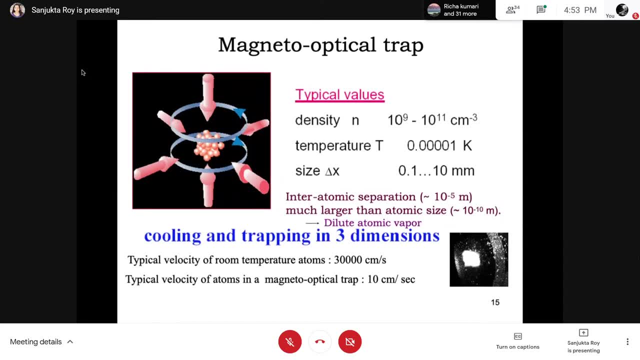 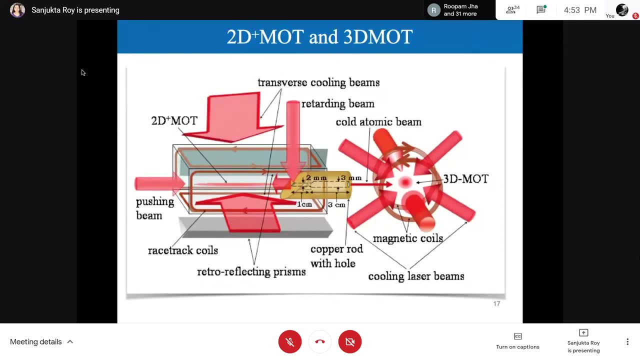 a typical velocity of atoms in a magnet optical trap is like 10 centimeters per second, so they are really cold and at very low temperatures. so how do we actually realize that? now? uh, just to start with our uh experiment in tifr, where we had actually realized the first bc, uh, we, uh, we had to adopt a very specialized strategy. 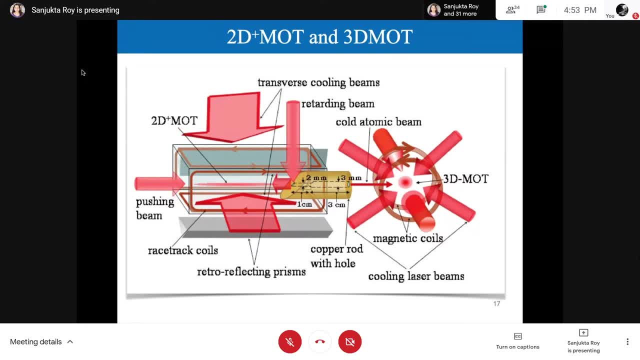 to have as much number of atoms in our trap because, uh, as i will show in in the in next after a few slides, that the actual- i'm an actual- process of getting to the bc. uh in it involves something called evaporative cooling, which which includes loss of atoms, so we wanted really to start with a very large number of atoms. 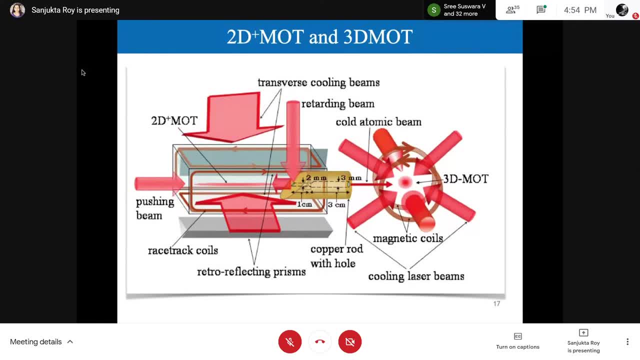 uh, after it. so we, uh, we have. we had designed a special trap called a two, two-dimensional magnet optical trap, which is actually called a 2d plus magnet optical trap, which is trapping in two dimension, in the transverse direction, but cooling only only cooling in the third direction. so you, 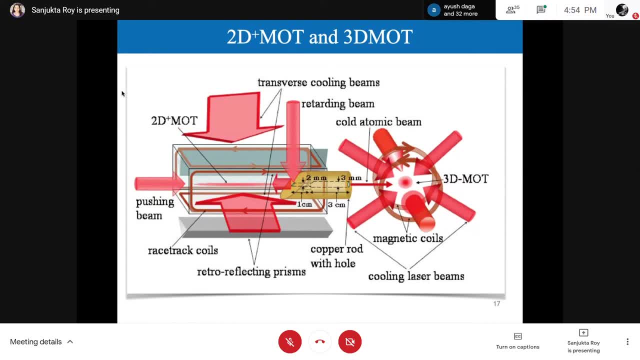 know, uh, the transverse variation does not travel, killed the Juice element, when in fact what cares about is the heat of the система, energy they actually abets, obviously the pressure of the host vapor of air. so you think about something like the size at eu kolis: a one woman's body. 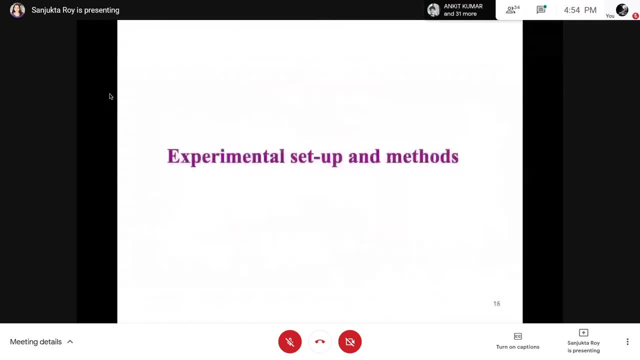 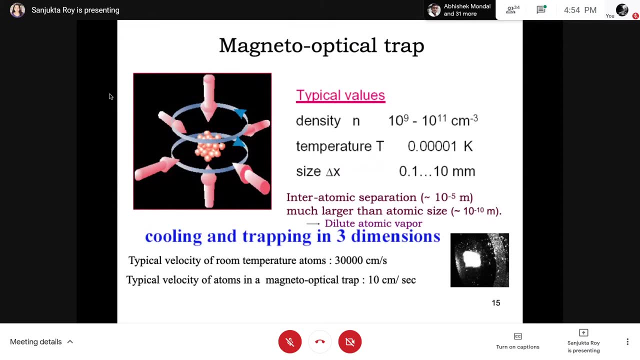 there is a mass of calcium and that has a specific reaction, which means the charge that foil of the Current emits telepathically. um means that as the air enters the earth a power lamp sells ça often gets absorbed by the air and causes a kind of environmental imbalance like the 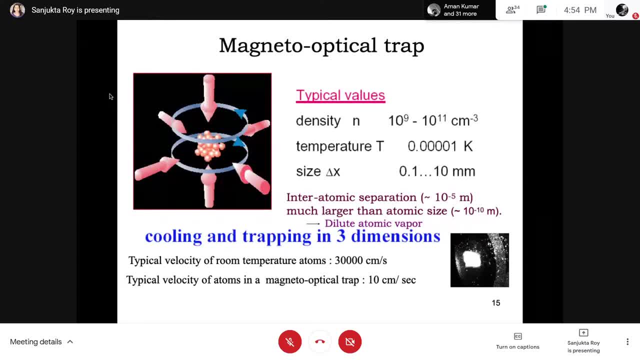 Mindkiw, pressure of the Earth increasesifies itself. or there are, you know, rectangular magnetic coils which isло rêu, Uh, middle entender, pressure like around 760 torr, and we need the vacuum inside the vacuum chamber to be around 10 to the power minus 11 torr. So it's like, really, you know, 10 to the power, 12 orders of magnitude. 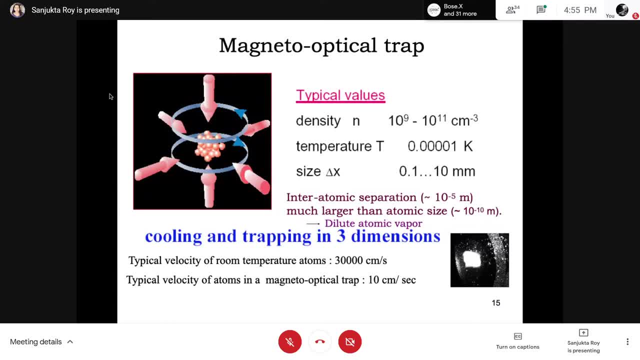 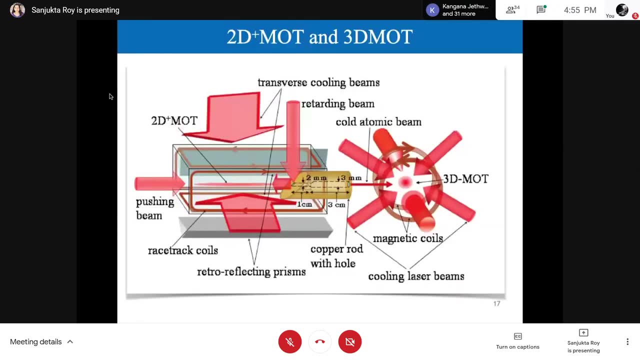 you know, lower at pressure as compared to the atmospheric pressure. This is because we don't want the hot atoms to actually knock out the very, very cold atoms in the magnetoptical trap, which is very low energy. So here we devised an experiment to actually realize a cold atomic beam. 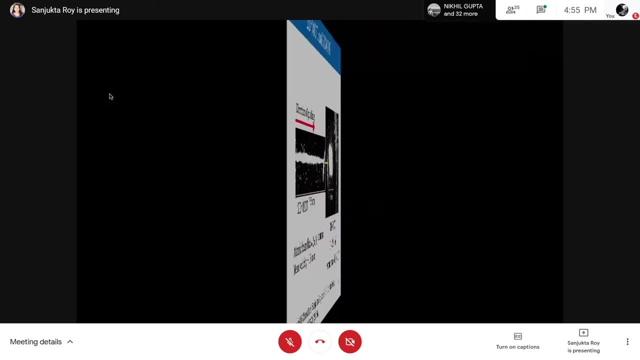 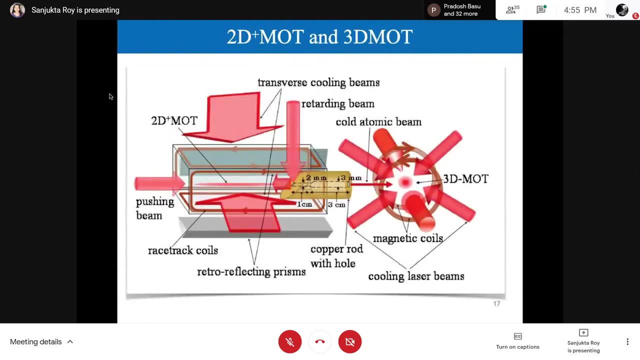 to load the 3D magnetoptical trap. So this is how we got. we did two-dimensional trapping in the magnetic trap. So this is how we got. we did two-dimensional trapping in the magnetic trap, the transverse direction and only cooling in the third direction. and then we actually- uh, we passed. 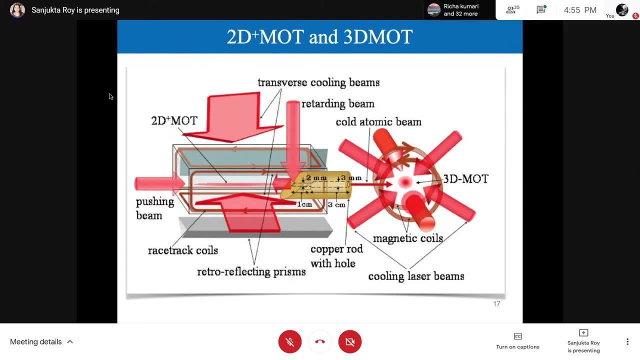 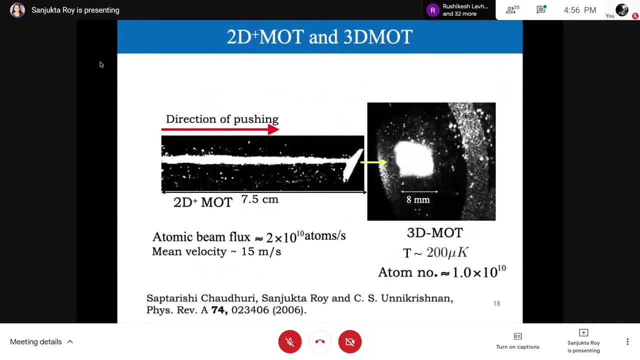 the cold atomic beam through a very us a cylinder with a very, very narrow hole and then this cold atomic beam could pass all the way through the tube to load a 3d of 3d magnet optical trap. so this is a picture of the cold atomic beam which we realized and then we it could. uh, it was a very 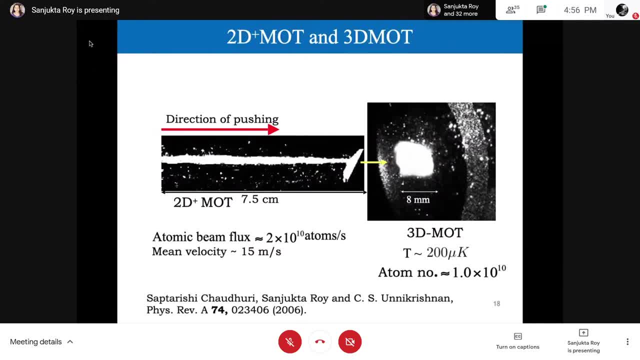 successful experiment, and this actually was one of the initial main reason. we could realize the whole seinstein condensate with a good atom number. so here we uh have produced the cold atomic beam which loaded a 3d magnet optical trap and we could get a cold atomic beam with very high flux. 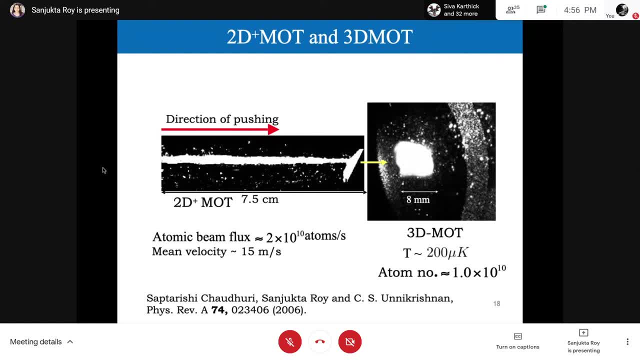 of 10 to the power 10 atoms per second and we could get a very, very large magnet optical trap with 10 to the power 10 atoms. so this experiment, this design for a 2d plus mod, was actually uh followed in many uh other labs in the world who wanted to make uh. 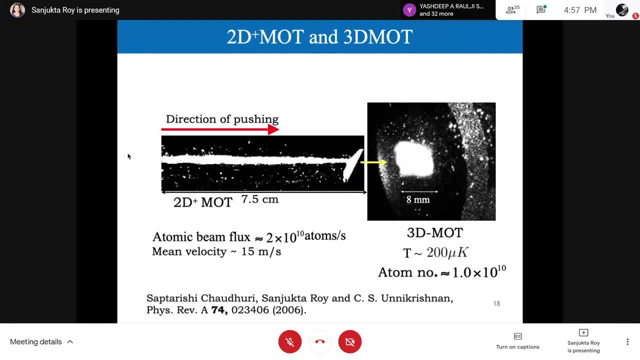 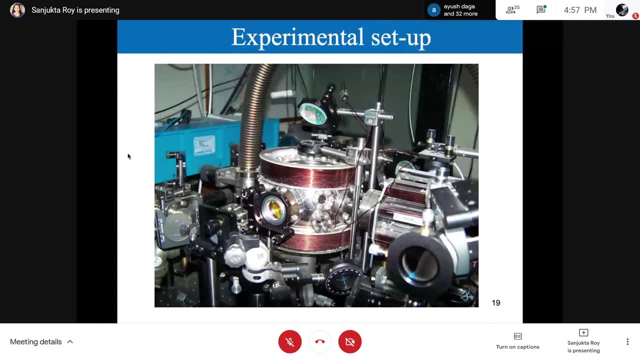 realize an experiment for bc starting with a very large number of atoms. so this is actually the photograph of our experimental setup. so on the right you see uh, the, the vacuum chamber for the 2d plus magnet optical trap, and then on the left, you see the bigger, uh the, the cylindrical, i mean the. 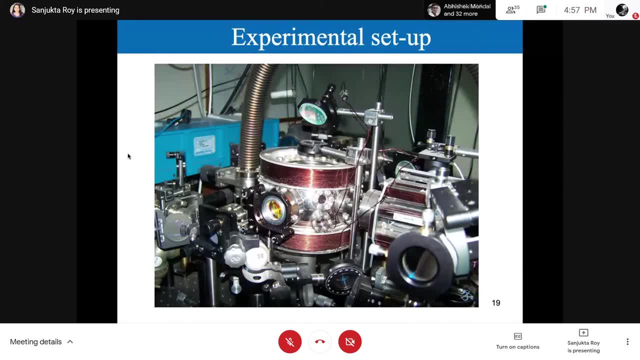 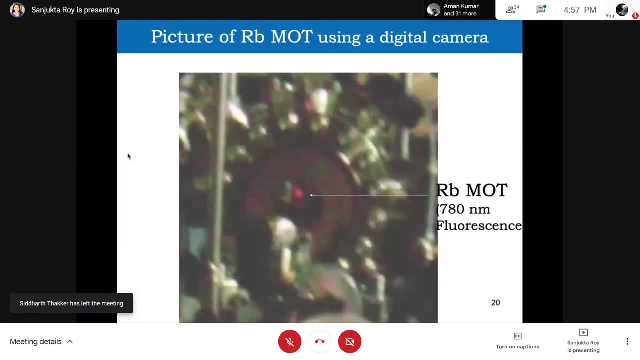 cylindrical vacuum chamber where actually the 3d magnet optical trap was produced. so we had a very large magn um number of atoms in the magnet optical trap so it was emitting a lot of fluorescence that we could actually see the atomic cloud with um directly, uh, without using a ccd camera. 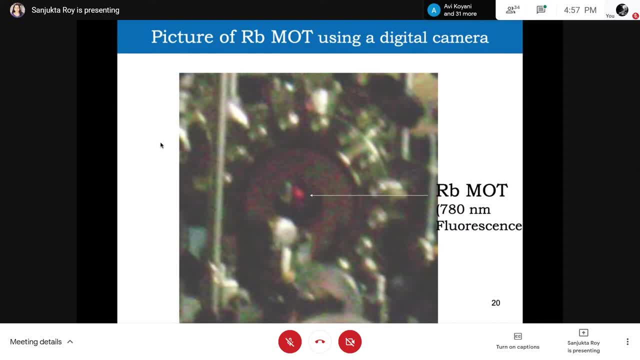 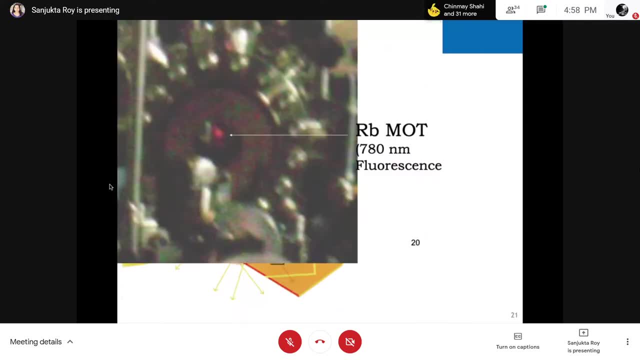 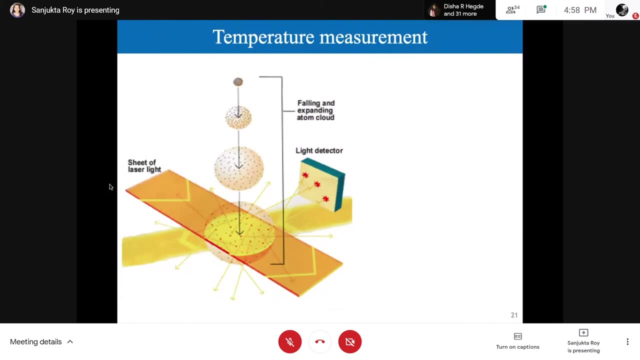 so here we see, you can see this red robera mod uh directly, which was using uh, taken using a digital camera, a normal digital camera. so you must must be wondering how to we say that, okay, this is the temperature of the cold atoms. we actually cannot place the thermometer inside the vacuum. 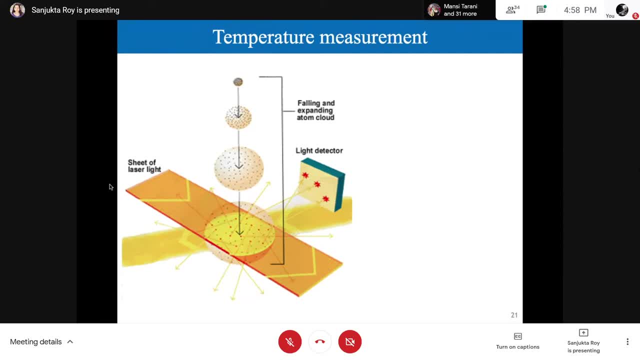 chamber but we have our special uh methods to do the temperature measurement. so what we do is we release the trap. we release, we switch off the magnet optical trap and let the atoms fall and expand now faster. i mean, the higher the temperature of the atoms, so the higher will be the momentum. 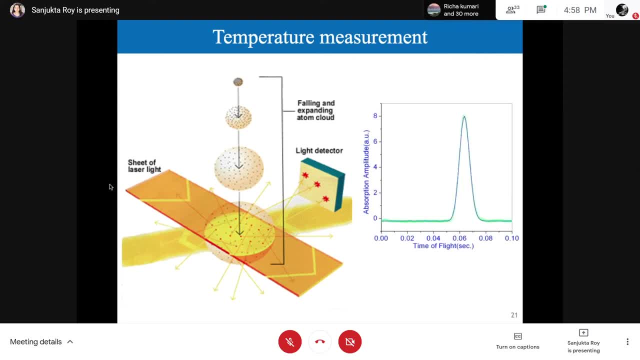 of the atoms and the faster it will expand. we probe the expansion of the atoms using a probe light and have the probe light on the detector and from the width of of this atomic density profile or how much it has expanded in a particular period of time, you can from the 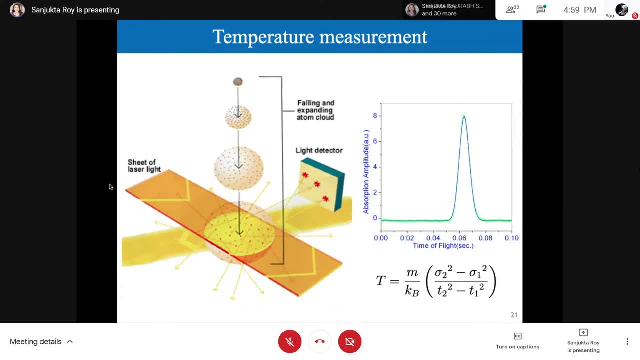 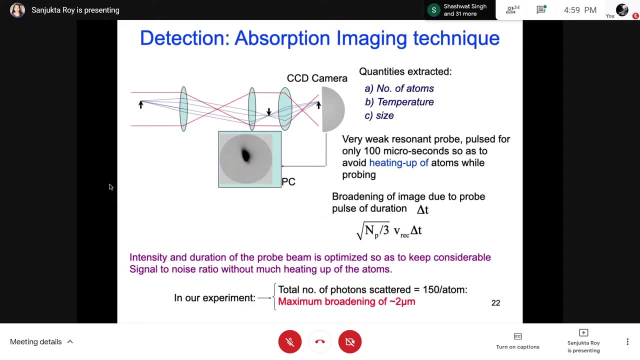 width, we can actually know what is the temperature of the atoms. so how do we actually see the atoms? we see the atoms by using absorption imaging. so we pass a probe beam which is resonant to the atomic transition through the atoms and then we image the shadow of the 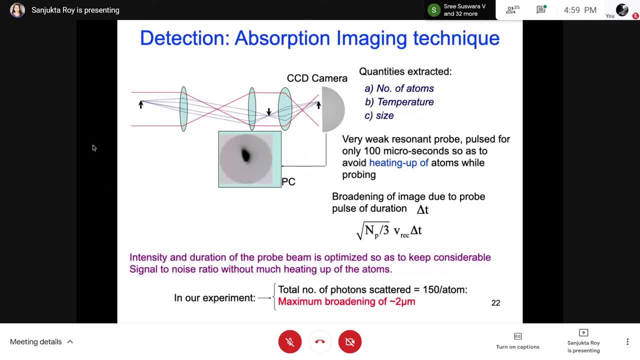 atoms in the probe beam on a ccd camera. so that's how you can see that this dark part you can see is actually the shadow of the atomic cloud imaged on a ccd camera. so that's how we detect the detect the atomic cloud, and from the, from this absorption image, we can extract all the. 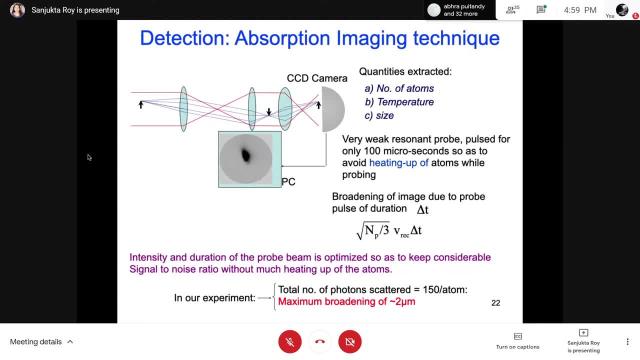 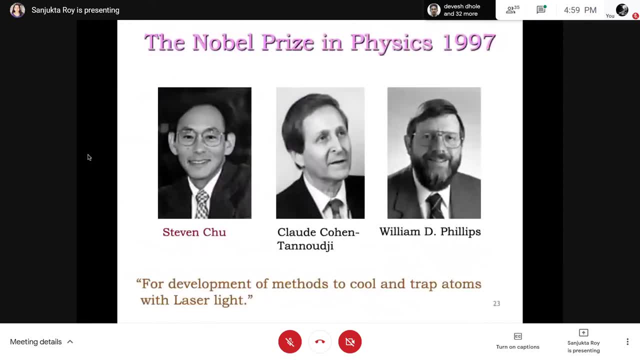 necessary information we need for the atomic cloud. we can know the number of atoms, we know the temperature, we can know the, of course, the size of the atomic cloud. so for laser cooling and trapping, which i have described till now um the three great uh physicists, steven, chu, claude, 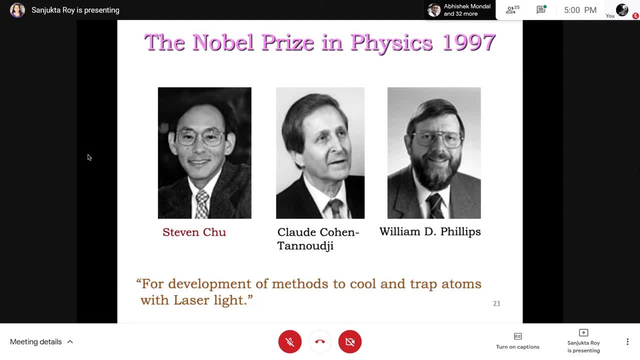 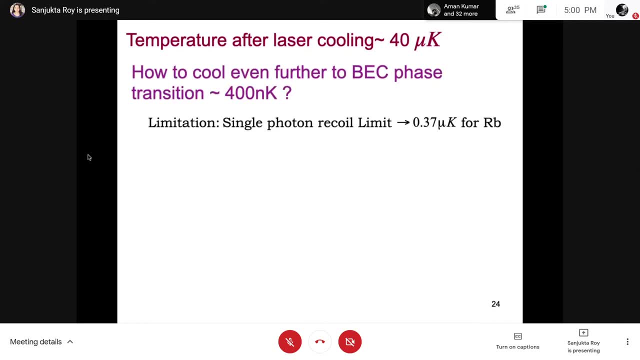 phillips, he they got the noble fries in 1997 to develop methods to cool and trap atoms with the with laser light. so now, as we saw that the lowest temperature we can get by laser cooling is like around 40 micro kelvin, now how to cool even lower. 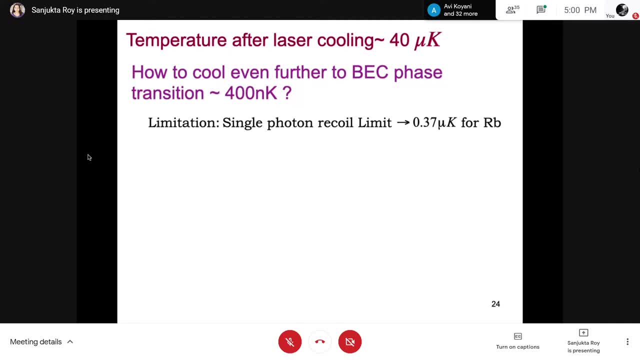 to go to bc phase transition. so we need around few hundred nano kelvin to go to bc phase transition. so we need to cool further. now you may ask: okay, we laser cool further and go there, but it's not possible because of something, a limitation called the single photon recoil limit. now, as i said that, 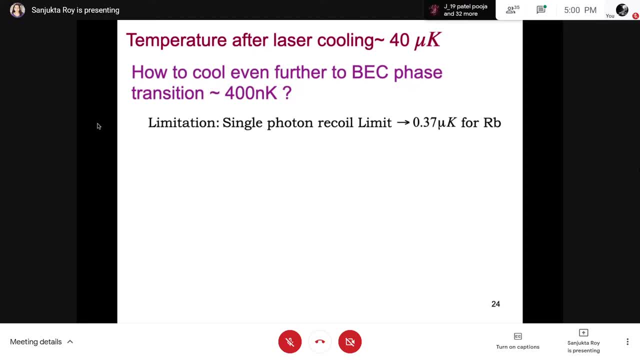 these photons which are used to cool down the atoms. they are on resonance, but these are also because of spontaneous emission. they also cause a little bit of heating of the atoms. so the heating by a single photon absorption of the atoms will cause a little bit of heating of the atoms. so the heating by a single photon. 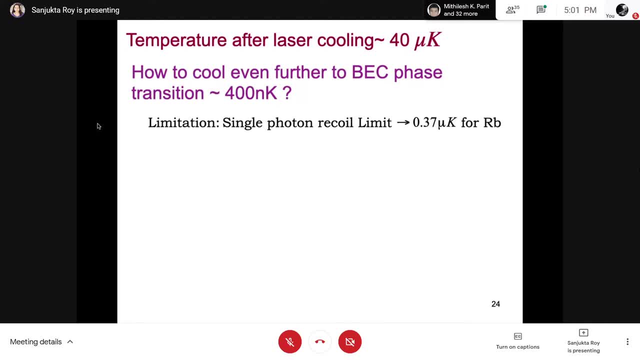 by the atom is like around one micro kelvin of the order of one micro kelvin. so we cannot actually go below one micro kelvin because if we are having uh resonant photons to cool we we cannot go below that uh temperature. so we need something where we don't have any absorption of any resonant photons. 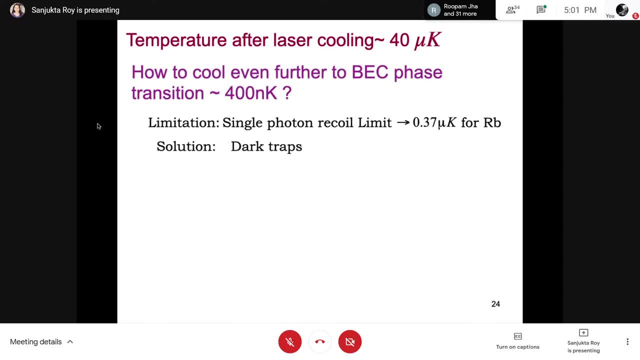 so we need something called a, called dark traps. so there are two kinds of dark traps, which is like absence, of absence of resonant light. so we have two uh kinds of dark traps where we do the next step, uh, for going to the bc, which is the evaporative cooling. so the options are magnetic trap. 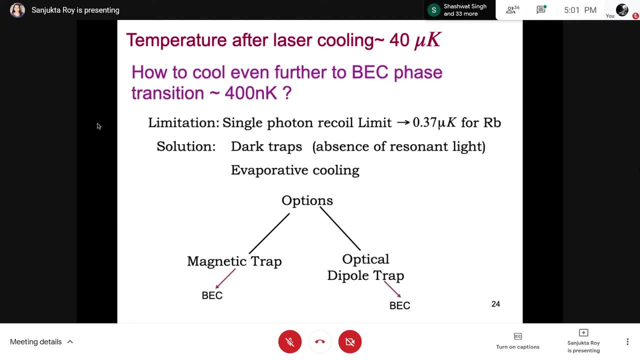 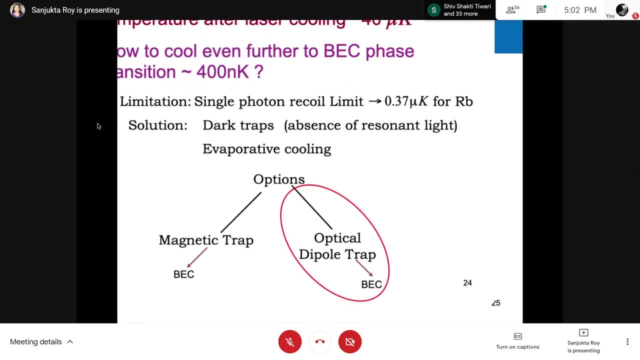 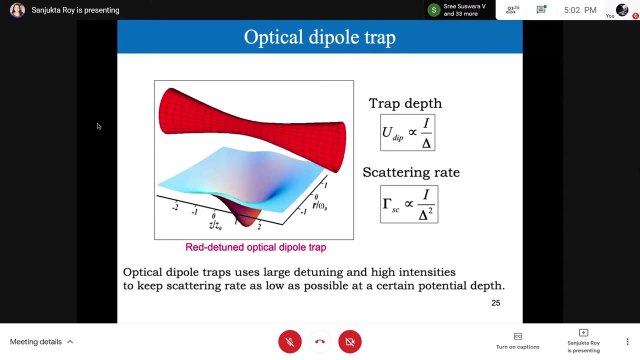 option is the optical dipole trap now. so this is what we had adopted for uh going to the bc, uh at tfr. so what is an optical dipole trap? so if you have a very high power laser, very, very uh, whose frequency is very, very far away from the 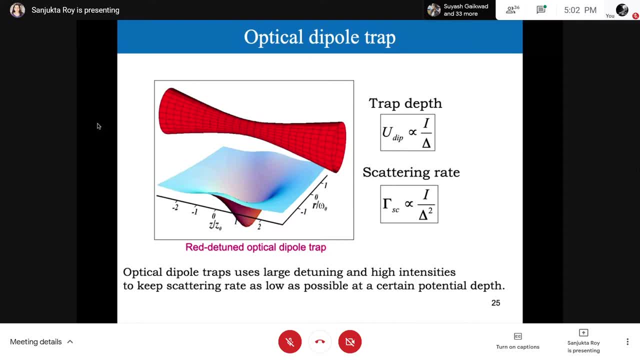 atomic transition, so that there is no absorption of the photon to heat up the atoms. uh, if you focus the laser beam at the point where you have the atomic cloud, it actually creates a potential for the atoms to be trapped. so the potential, the depth of the potential is: 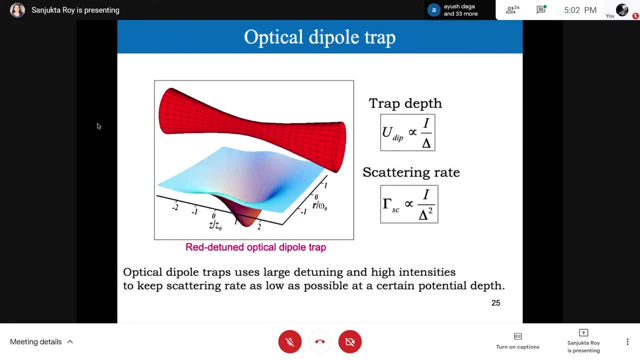 proportional to the intensity. that means higher the intensity, which is the largest at the focal point. the higher the intensity, more is the potential depth and the more number of atoms you can trap and larger is the detuning. that means you can see that the detuning, which is the delta, is in. 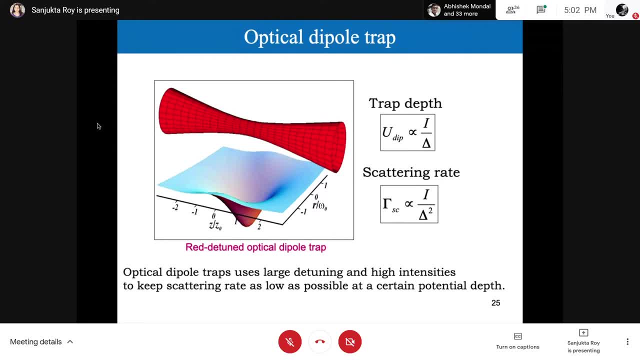 the denominator, so the larger the detuning, so lower will be the scattering late rate. that means lower will be the heating. so we use very high power lasers with very high intensity and very, very far uh بتhe, expanding the decomposition and this is. you can see that this is can be. 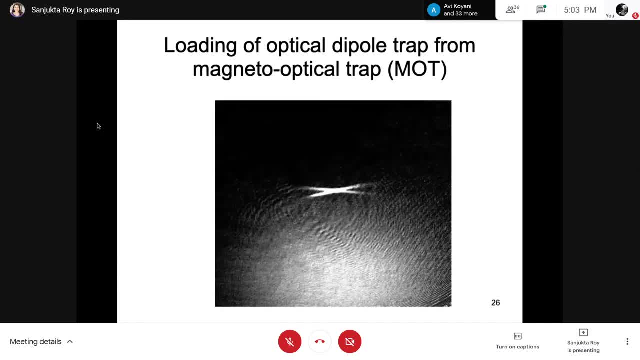 easily adjusted. if omega t times beta is at 100 and even below is ach allows you to appreciate, uh, the peak volume here. okay, okay, take a look here. um, the ripple trap they are. you know they are getting lost as we switch off the bandit optical trap. 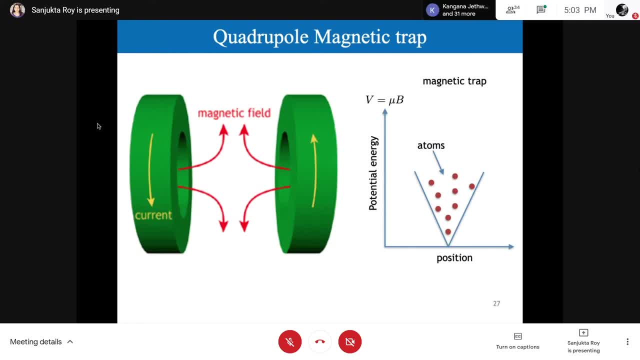 another way actually to uh trap the atoms in a draft trap which is using a magnetic trap. so we use a quadruple magnetic field with the currents in. we have two uh coils in anti-hell balls configuration with currents in the opposite direction, so which creates a zero. 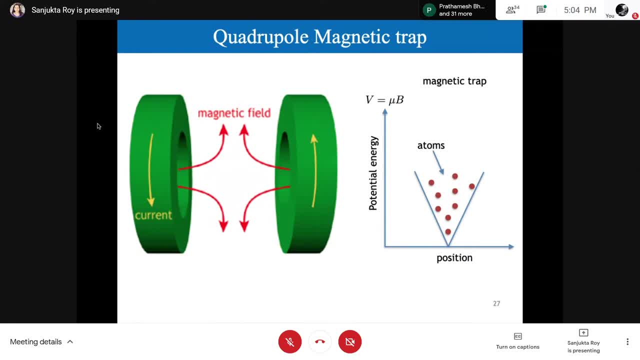 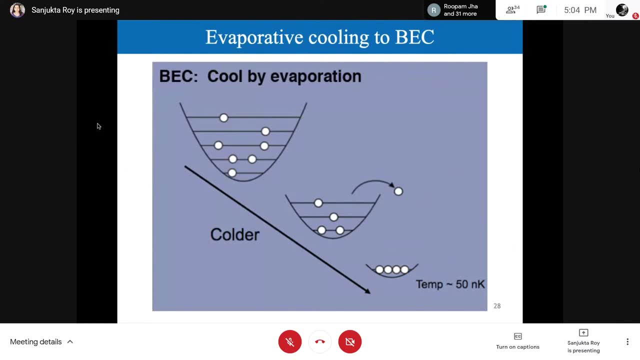 at the center and it increases linearly in all directions. so that creates a magnetic trap where you can actually trap the atoms. now the very important step to go to the Bose-Einstein condensate is something called evaporative cooling. so how do we do that? so, once the atoms are trapped, 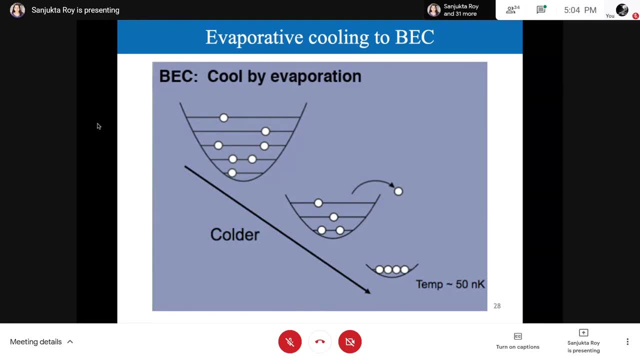 in in the in one of the traps. so what we do is we lower the depth of the of the trap. so here, when the atoms are actually trapped in a in a harmonic trap, the higher energy atoms are actually at the outer region of the trap and the lower energy atoms are actually at the center of. 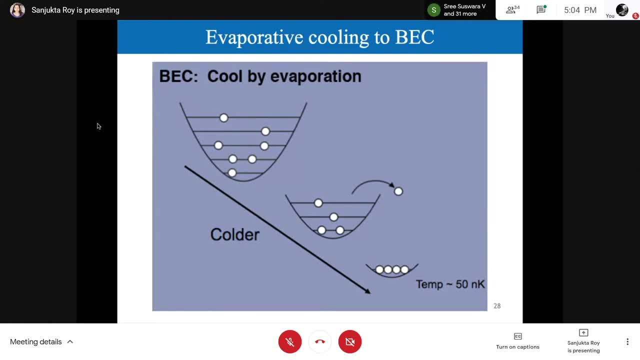 the trap. so when we lower the depth of the trap, the hotter atoms which are at the periphery of the trap they get lost and get evaporated away from the trap, and the lower energy atoms they get, they actually elastically collide among themselves and then they overall and then then they lower the overall. 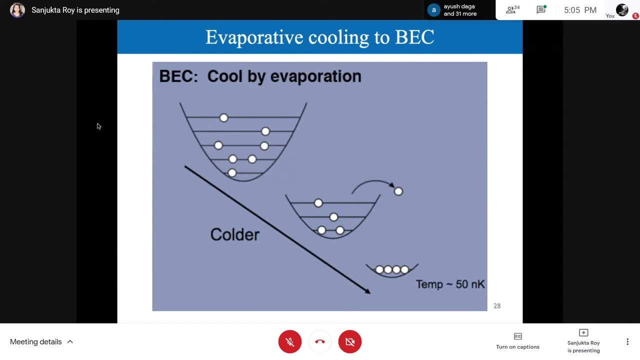 temperature and get cooled step by step. so this is like actually cooling off your coffee cup, where the hot atoms are getting evaporated from the cup and the lower and lower energy atoms are actually uh colliding and then it's reducing the overall temperature of the system. so after you lower the 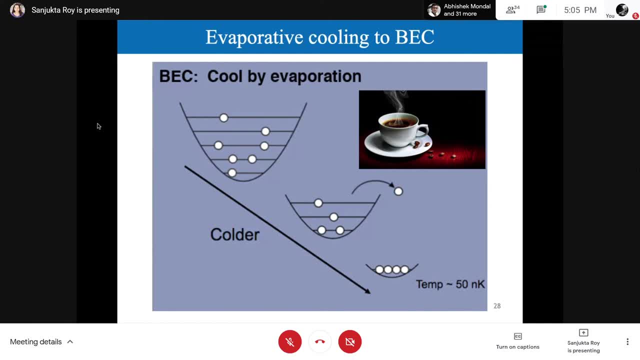 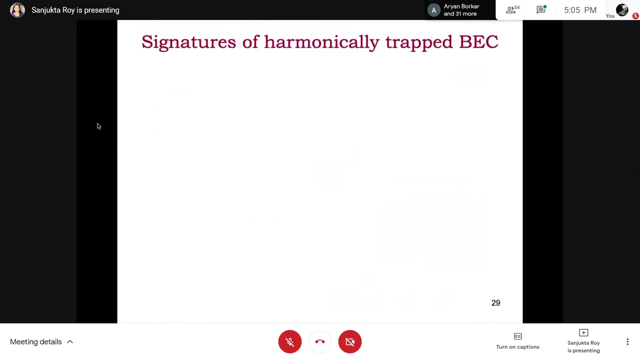 atoms, step by step you go down and which actuallyscaps also one that to go to a very low temperature and actually cross the BEC transition temperature to get all the atoms at the lowest momentum state of the trap and thereby reach the BEC phase transition. 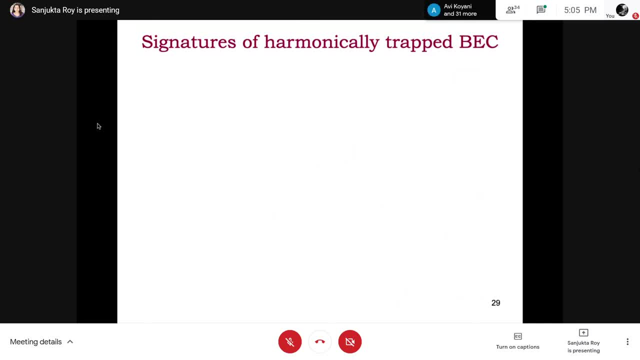 So how do we know that we have a BEC? So we need to have some smoking gun evidence or the signatures of a BEC. So one very good, harmonically trapped BEC is that the Bose Einstein condensation occurs in both position and momentum space. 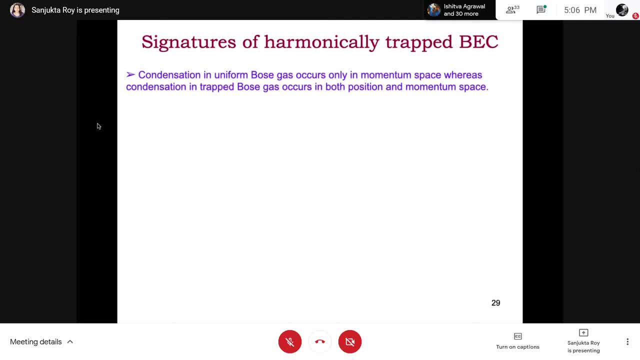 That means the higher momentum atoms are really at the periphery and the lower momentum atoms, or the coldest atoms, are at the center of the trap. So how do we realize that the BEC transition temperature has been reached? So it is observed as a sharp peak in the atomic density profile which emerges at the center. 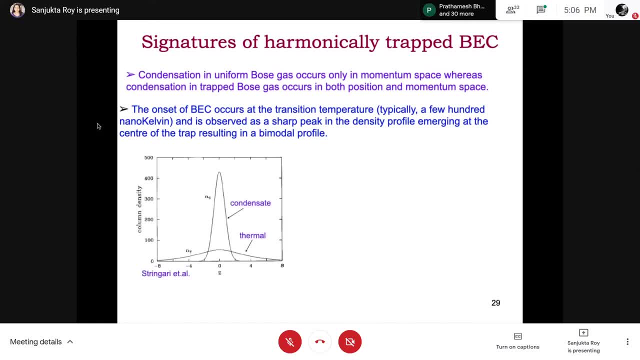 of the trap which results in a bipodal profile. So you will have a periphery of atoms which are not in the condensate- we call them thermal atoms- and we have the Bose Einstein condensate at the center, The atomic density profile from the BEC in 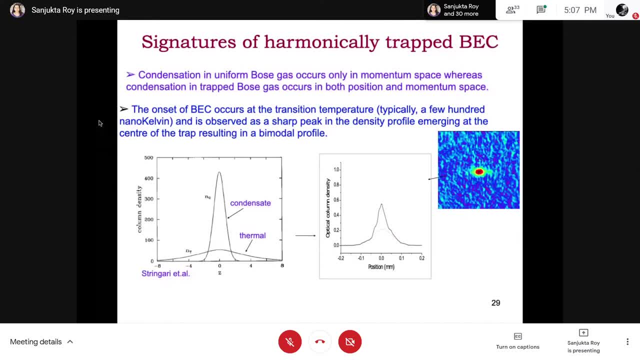 which we had realized at TFR. So here you can see that there is a broad profile of the thermal atoms and there you have a sharp peak which correspond to the dense atomic cloud at the center, which is the Bose Einstein condensate. So the coexistence of condensate and the thermal cloud is a characteristic of BEC in a harmonic 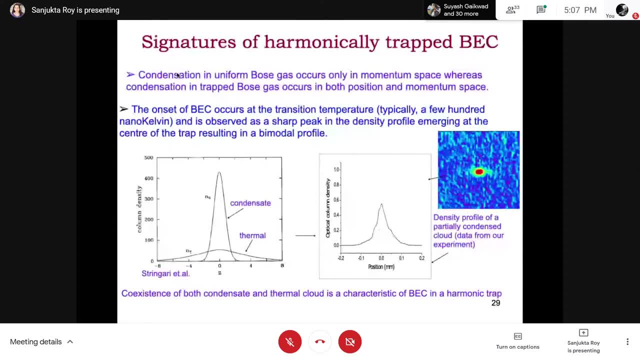 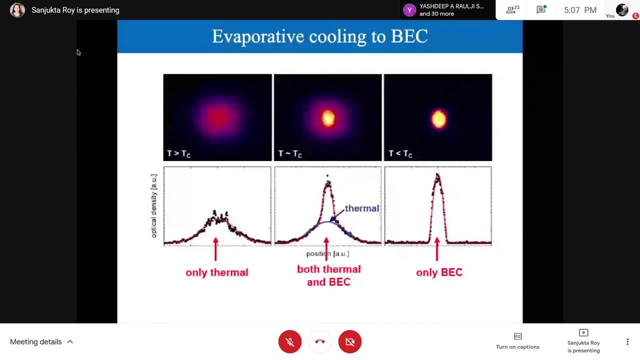 trap and also the smoking gun evidence. So you can see that when you have not a temperature, where you have high temperature, there you have only thermal atoms. but when you have reached the BEC transition temperature you have a coexistence of the thermal cloud and the Bose Einstein condensate, which is a sharp 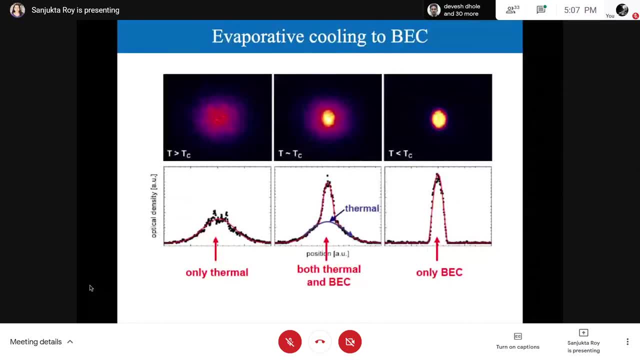 peak at the center and as you lower the temperature further, you have only the Bose Einstein condensate. So how to explain this? So we have this parabolic profile which is the characteristic of the Bose Einstein condensate. So this has to do with the interaction of atoms in the Bose Einstein condensate. 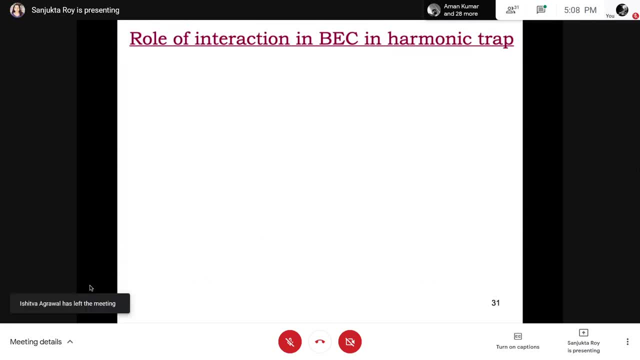 Now how do we explain the atoms in a Bose Einstein condensate in a harmonic trap, Train it using a Gross-Petrovic equation, which is actually a non-linear Schrodinger equation. So it is actually consists of a kinetic energy form, The term for the external potential, and we have our interaction term mean field interaction. 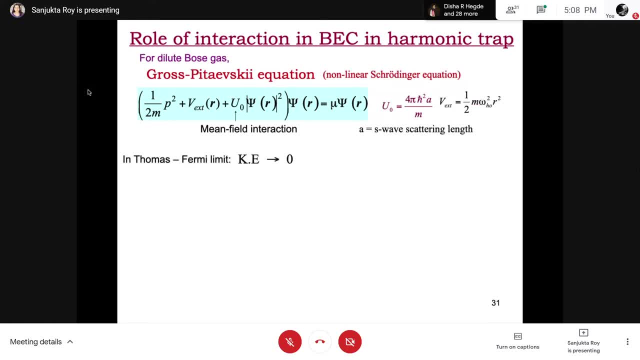 Now in the thermos Fermi limit we have a limit where the kinetic energy is zero because the atoms are very, very cold. We have the atomic density profile, which is actually gives the shape of a parabola. So that actually explains why you have a parabolic shape. 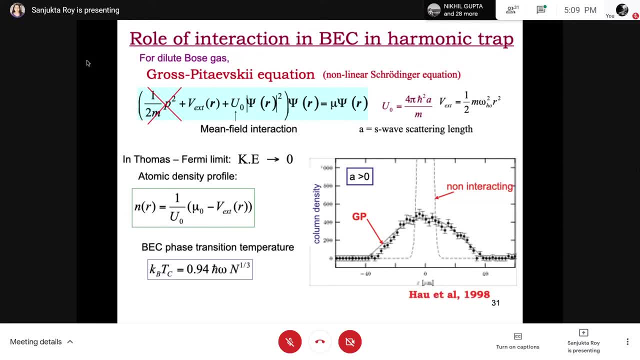 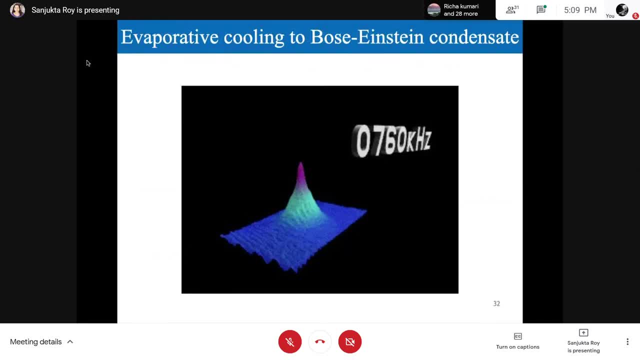 So the the density profile is shown at various stage of the BC. So here you can see a sharp density peak appearing at the center which is actually the smoking gun evidence of the Bose Einstein condensate. So here you can see a sharp density peak appearing at the center which is actually 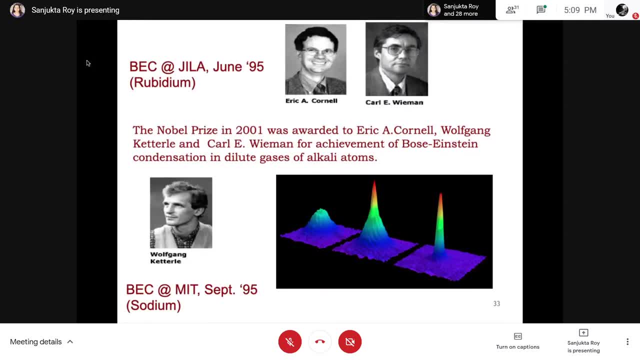 the smoking gun, evidence of the Bose Einstein condensate. So for producing, realizing the first Bose Einstein condensate in the world, So it was realized in Xela, in Rubidium, by Eric Connell and Carl Weiman, and in MIT by 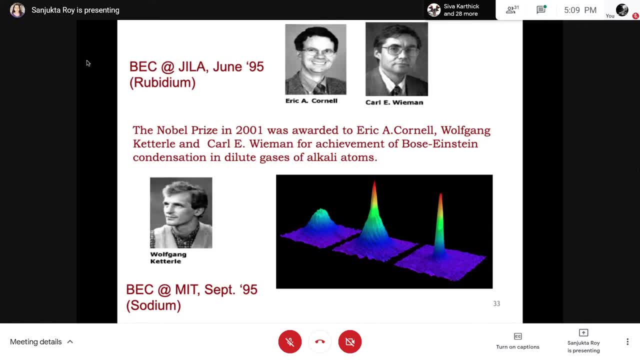 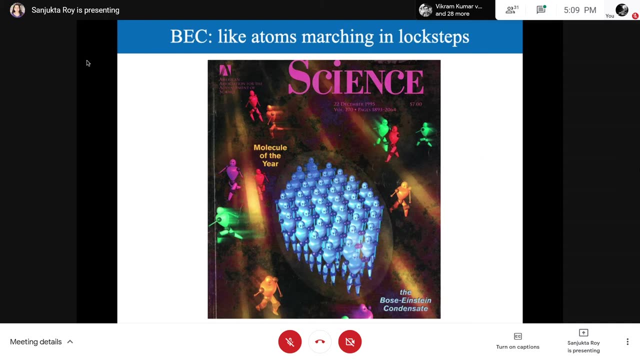 Wolfgang Ketterle, and they won the Nobel Prize in 2001 for achieving the Bose Einstein condensate in dilute gas of alkali atoms for the first time. So this is actually the cover page of the journal Science And the first reporting of the BC was, so here you can see that the BC was actually 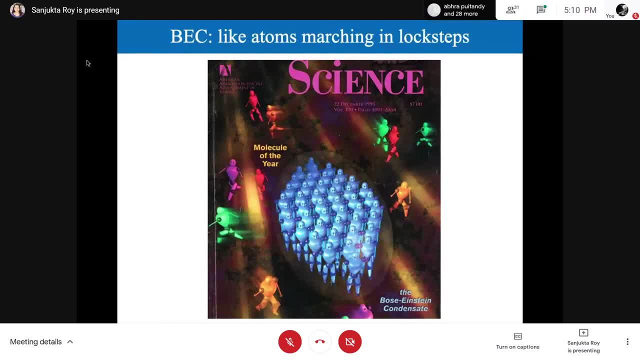 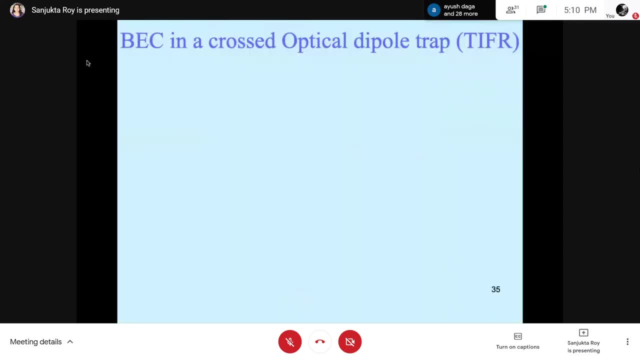 compared with the, with soldiers marching in lock steps. So it's like atoms marching in lock steps because they're all phase coherent. Picture of a BC in our in our TFR experiment, where we have before the transition temperature like at around 700 nanokelv. 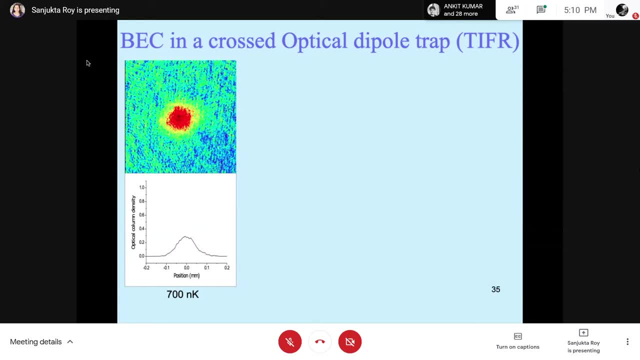 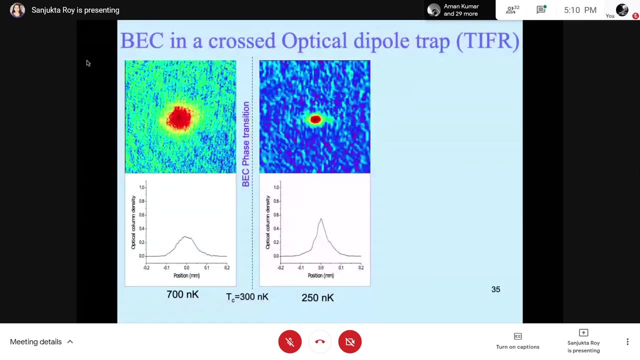 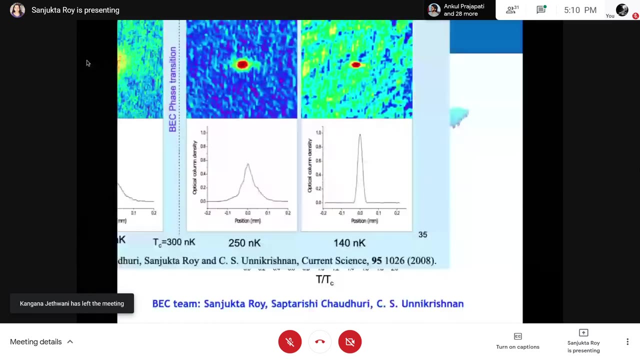 We have Fully thermal atoms And then we cross the BC phase transition and we see a coexistence of BC and the thermal cloud And then we have a pure Bose Einstein condensate as we go to lower temperature, our 3d profile. 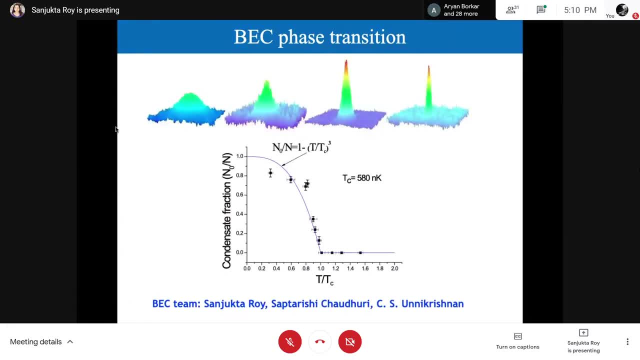 of the Bose Einstein condensate, And here the BC phase transition is is shown nicely in in this graph, where you see that before The transition temperature is reached The condensate fraction is zero, But as the at the BC phase transition that you see a sudden jump in the fraction of. 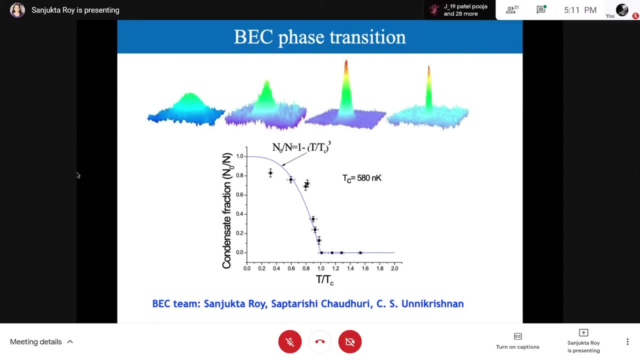 atoms in the Bose Einstein condensate BC team comprised of me and another PhD students at the Rishi Chaudhary and we worked under guidance of our supervisor, CS Unnikrishnan. So this is the picture of our BC experiment. 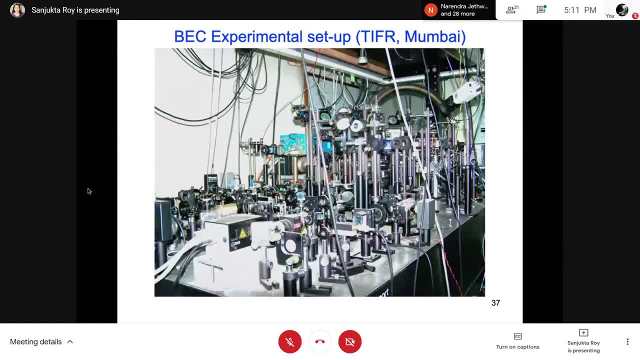 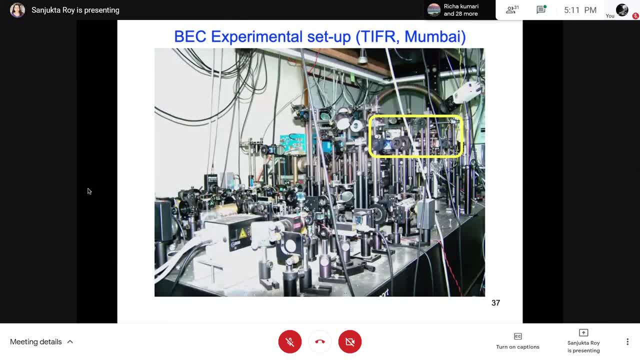 So here we have the place where we actually realized that BC and all the optics are actually to have the laser beams just at the correct, you know, amount, correct full ether, Individual and Intensity To actually realize the Bose Einstein condensate. well, I mean, it looks a bit complex. 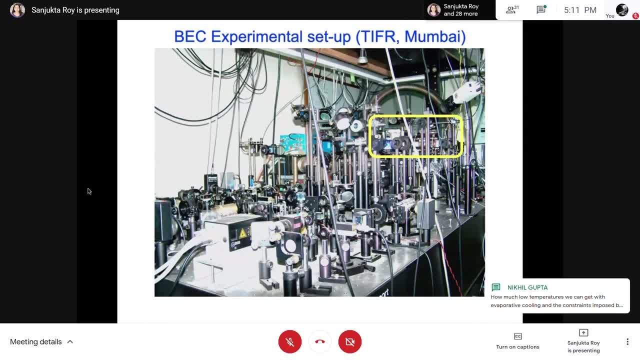 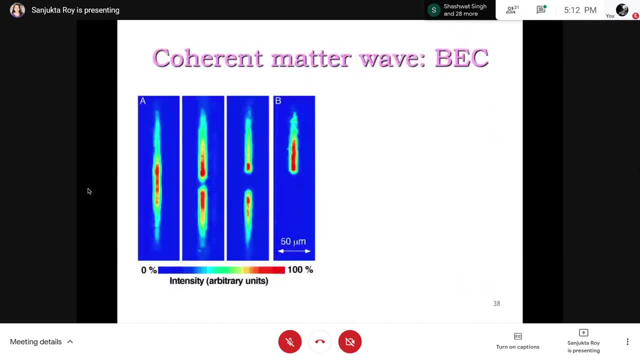 But when you actually see the nice in nature of Bose Einstein condensate on the CC d camera camera, you think that it's it's totally worth it. so, as I said that Bose-Einstein condensate is a coherent matter wave and the the smoking gun evidence for a 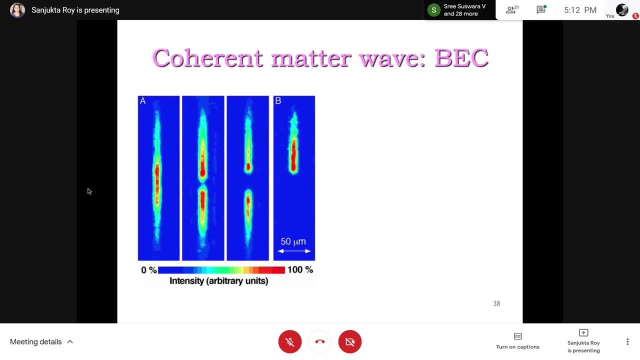 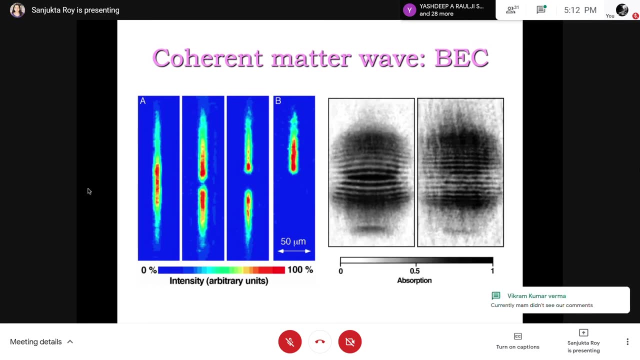 current matter wave is that it should be able to create interference pattern. so this is a picture of atom interferometry, a BEC atom interferometry in MIT, where the condensate was split into two and then made to recombine to get a interference pattern, which was actually evidence that the all the atoms in the 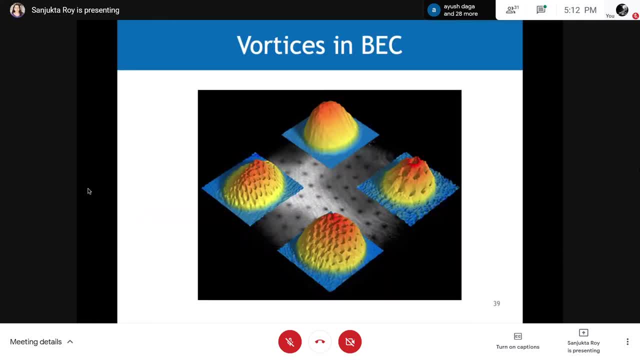 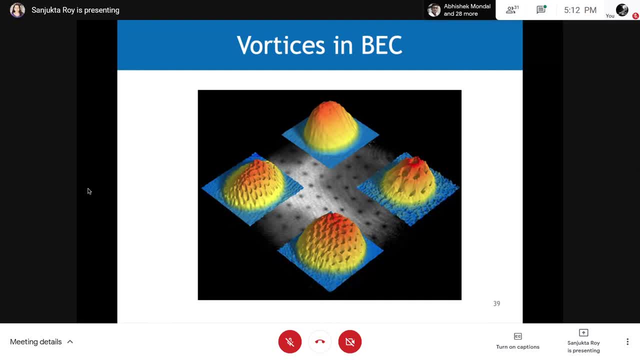 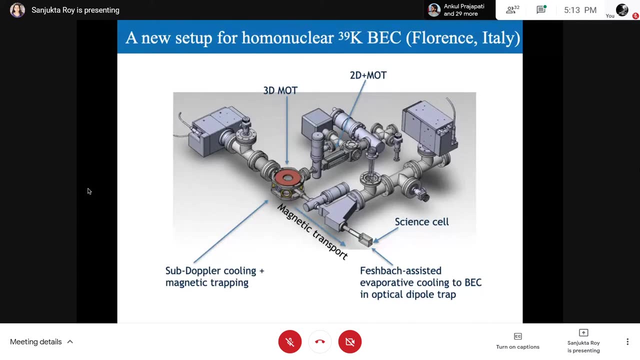 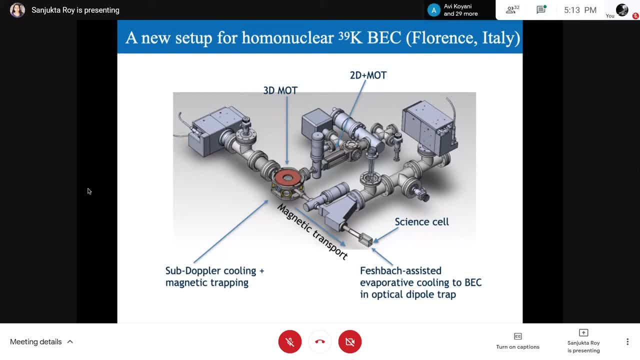 my postdoc in Florence. so it was. it is with the potassium, so till now I showed your BC of rubidium. so in Florence I actually built up a setup for potassium and it has a very nice advantage which I'll show you in a few slides. so we, as I said, our 2d plus mod design in many, many 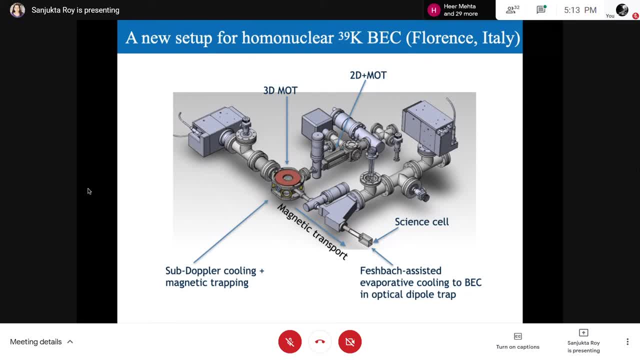 experiments in the world, and this experiment was also one of them which I had set up from the beginning. so this had a 2d plus mod and a 3d part, and then we actually magnetically transported the atoms from the 3d mod to something. 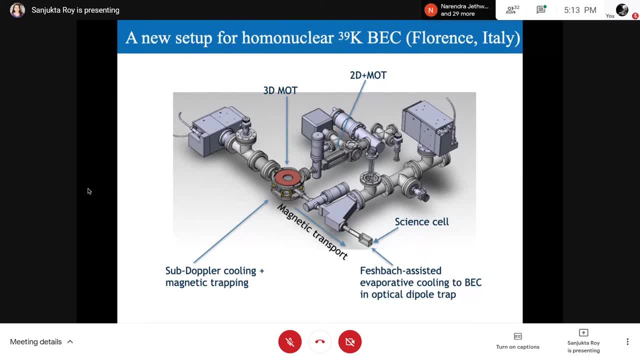 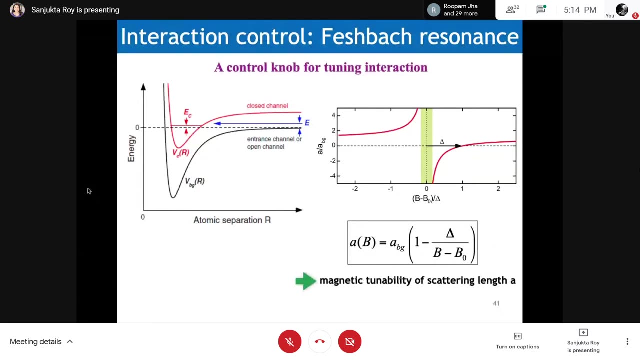 to a chamber called. we did all the science experiments. so potassium had a very nice property: that you could actually change the interaction between the atoms using something called a Feshbach resonance. so we changed the magnetic field and using what is called a Feshbach resonance we could change the 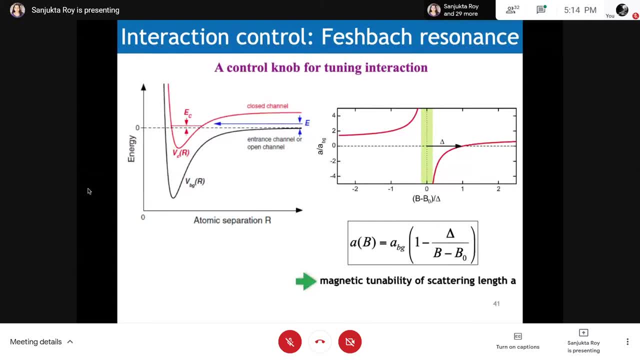 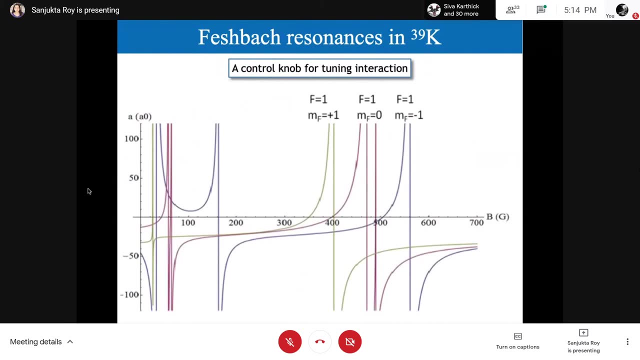 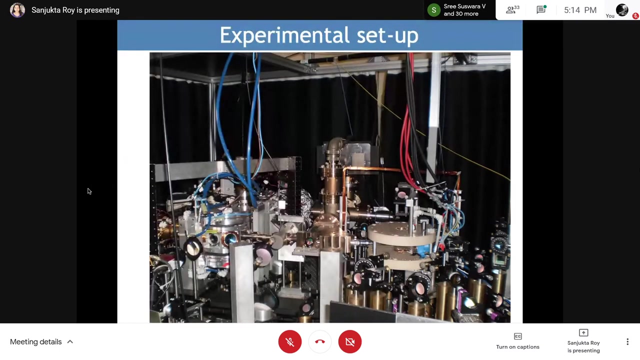 scattering length or the interaction of the atoms from, you know, minus infinity to plus infinity. so it was a very nice control knob for changing the interaction in the potassium atoms, a very large variety of Feshbach resonance by which we could control the interaction. so here is the experimental setup for our potassium experiment and 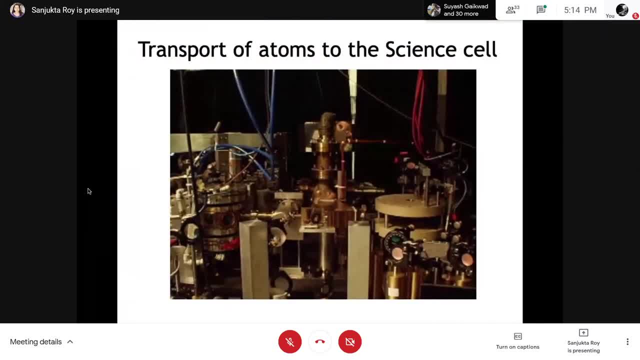 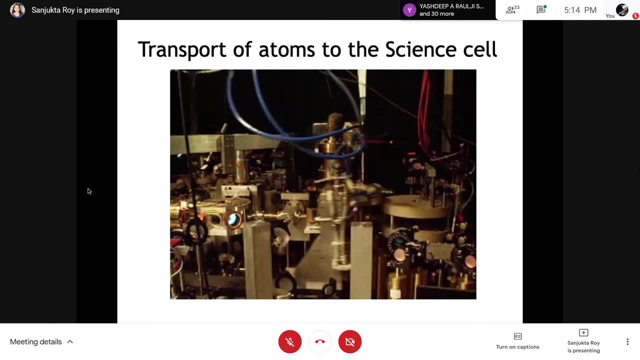 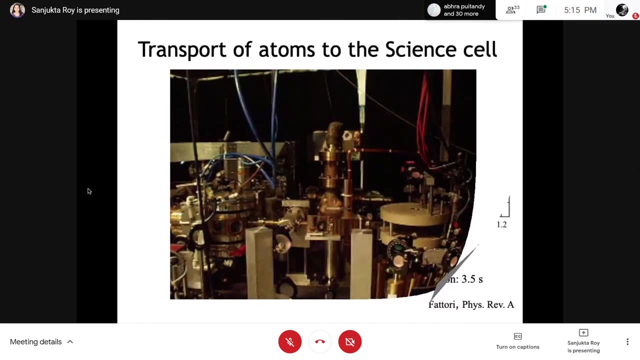 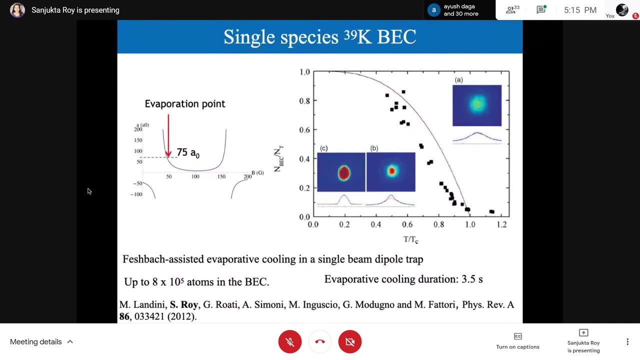 here you can see the video where, after producing the atoms in a 3d bond, we would transported magnetically into the science cell. so here is the picture of the Bเฉc phase transition in potassium. so this was actually the first single species BC for potassium, because in earlier experiments, since potassium had 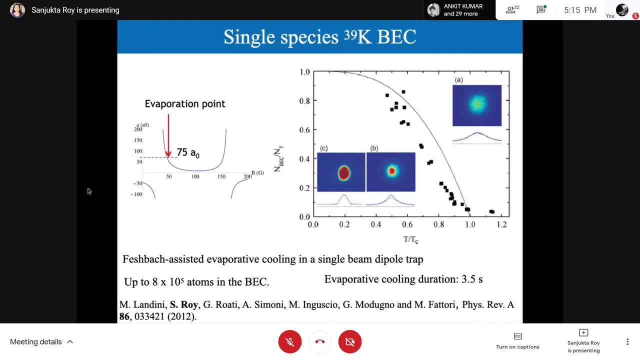 had didn't have any eggs yet, so the potential would have been higher than the potential had been higher than the potential would have been higher than the very favorable favorable scattering length for evaporative cooling. it had to be, you know, mixed with rubidium to get the BC, but here we have used fetchback. 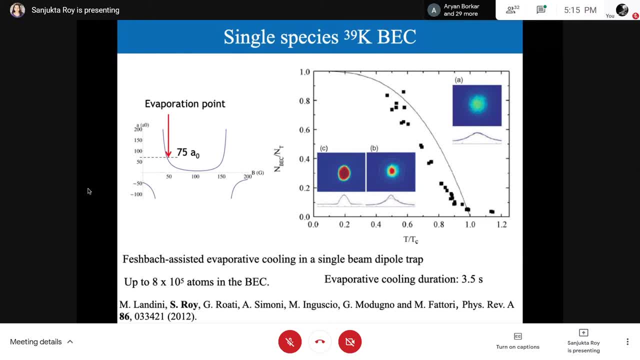 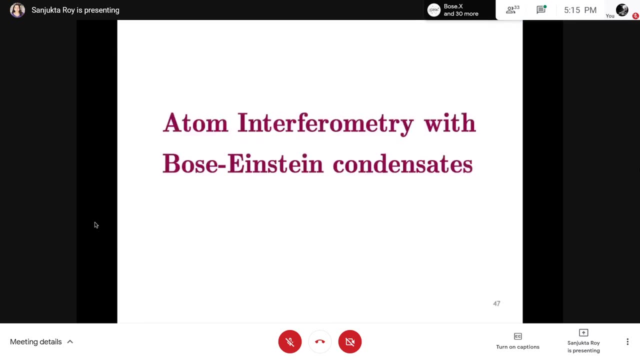 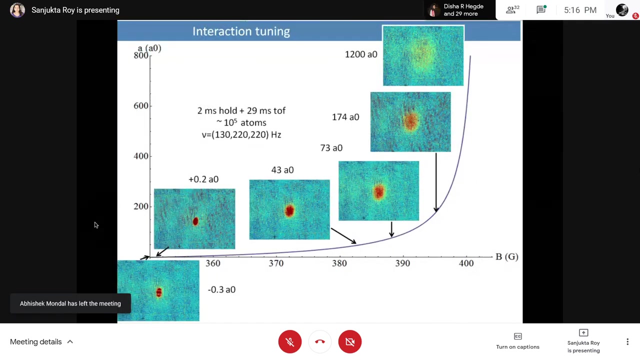 resonance to tune the interaction to a favorable quantity in the potassium to realize the BC. so it was for the first time we had a single species, potassium, 39 BC. so it was a very large BC with around 10 to the power 6 atoms. so here is the effect of the interaction. so then you can have either attractive 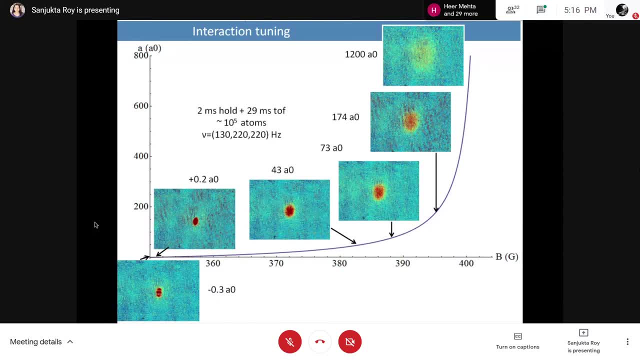 interaction or repulsive interaction in the BC. so when you have repulsive interaction, which we actually need for evaporative cooling to BC, you can see that as we are increasing the interaction, which is a, a, actually equivalent to increasing the scattering length of the atoms, you can. 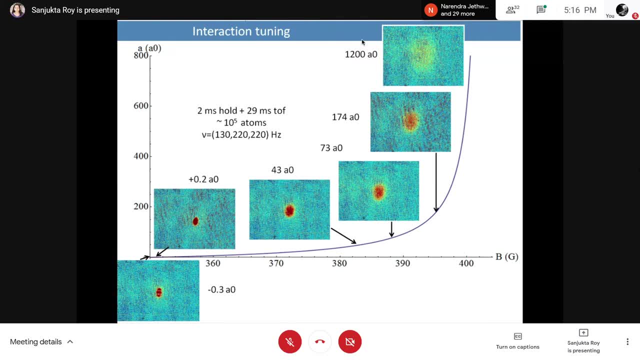 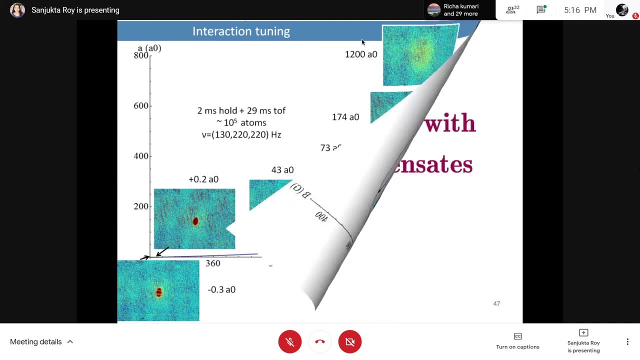 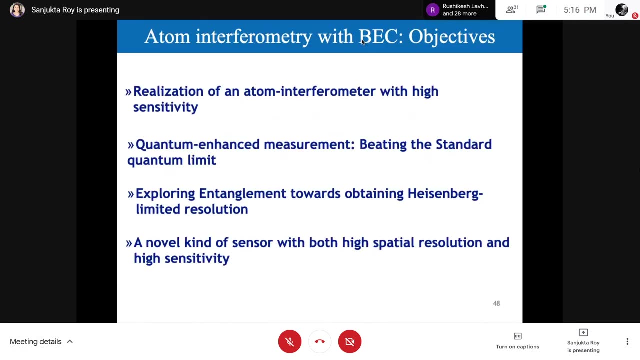 see that the BC, they're all in BC. they are getting larger and larger because of the repulsive interaction between the atoms in the BC. so we also did atom interferometry with Bose-Einstein condensate. so BC is a very useful atomic tool to do very precise atom interferometry and it can actually lead. 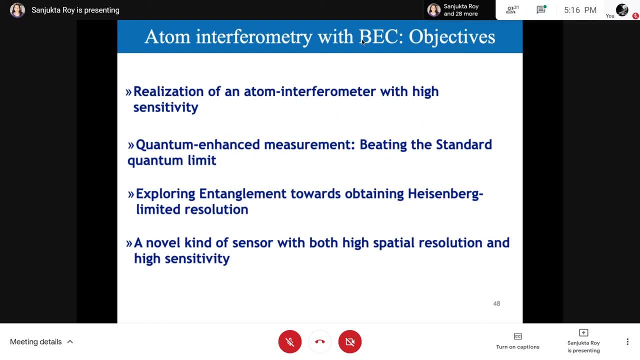 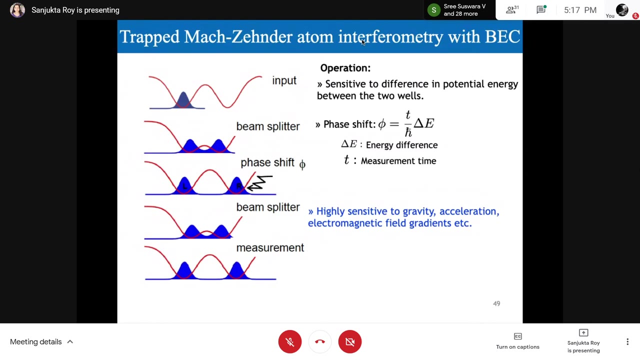 to quantum enhanced measurement, like beating the standard quantum limit, and also can realize entanglement between atoms and it can eventually reach the Heisenberg limited resolution. so it's a very high sensitive sensor with very high spatial resolution. so to get the atom interferometry we first produce a BC in a double well trap and then increase the spacing. 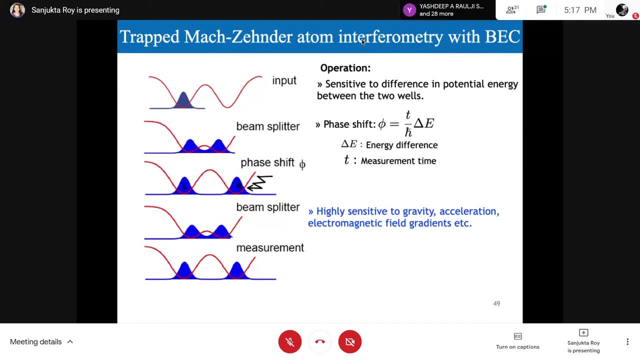 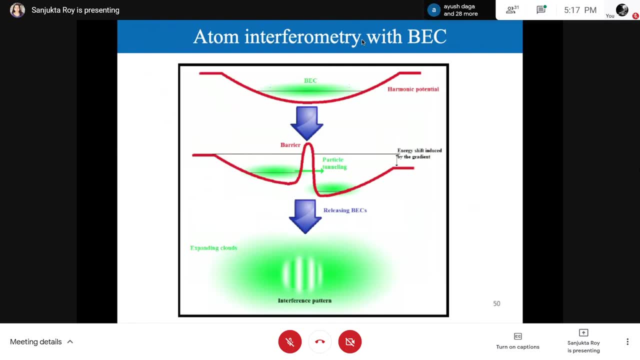 between we separated the BC and then we introduced a phase shift and then again recombine the BC to get the interference. so here we have the BC in a single trap and then we actually split the BC into two and then let it expand and recombine to get the interference pattern. so here you can see the 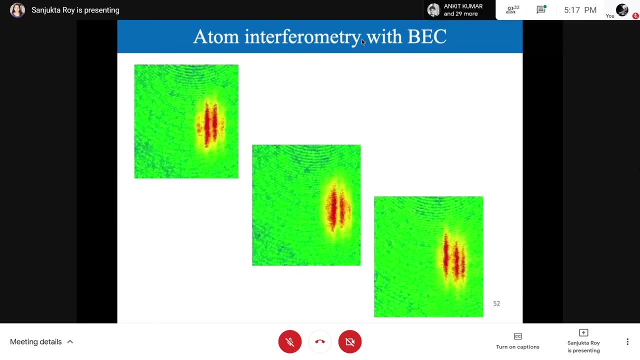 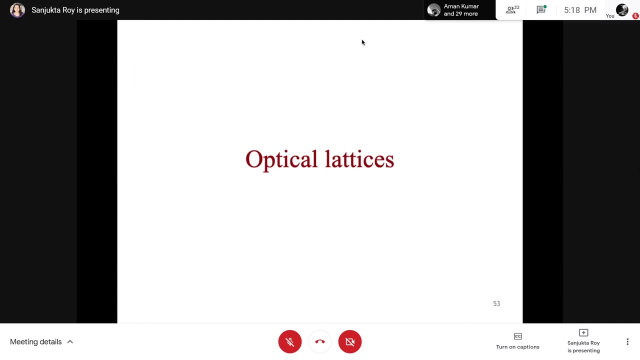 interferon pattern, and then you can see the interferon pattern and then you can see the real interference pattern of the BC after we split it and recombined. so it's a very useful tool for high precision atom interferometry. so next I move over to optical lattices. so optical lattices are actually artificial. 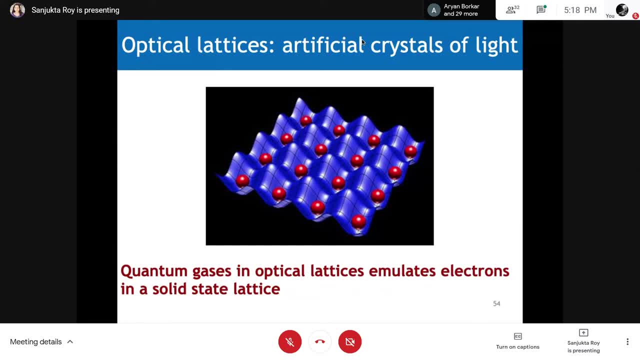 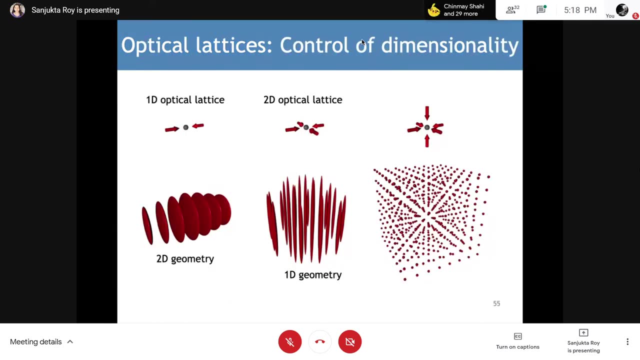 crystals of light and quantum gases in optical lattices can actually emulate or remnants of light. This allows Therapy and project: potematicобetsch straws and a small particle in a single wave to replicate a robbed layer ofсколько by COPYS, recordings and so on. 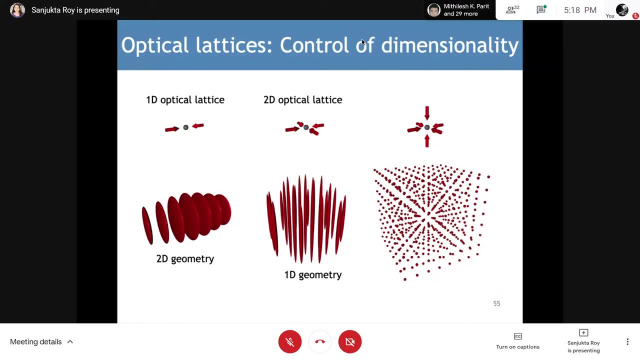 So here you can see. these are extrapolated assassins demonstrated in optical privilege. verme신 of the optical idea. lattice is a sort of pancake-shaped atomic cloud which are in a 2D geometry. Now, if you have 2D optical lattice, 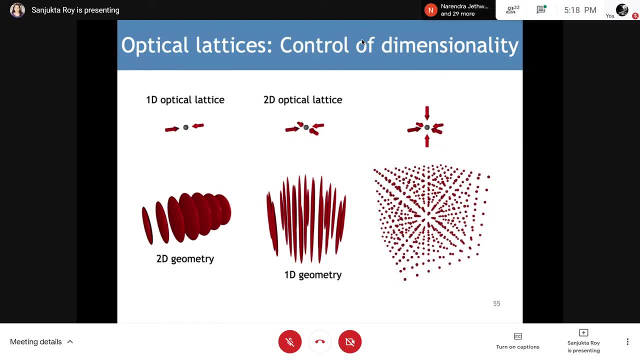 that means you have optical lattice in x and y direction. you get an array of 1D or rod-shaped atomic cloud And you can have also a 3D optical lattice. So here you can see that you can actually control very well the geometry of the atomic cloud. 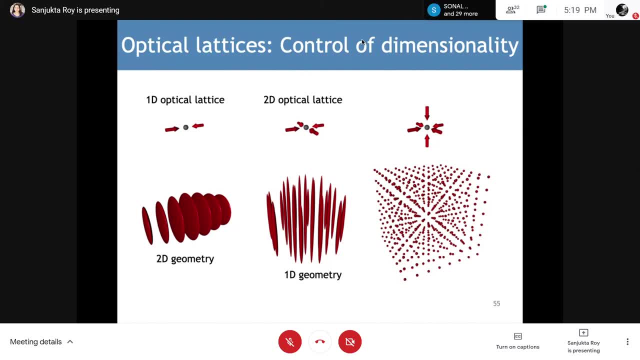 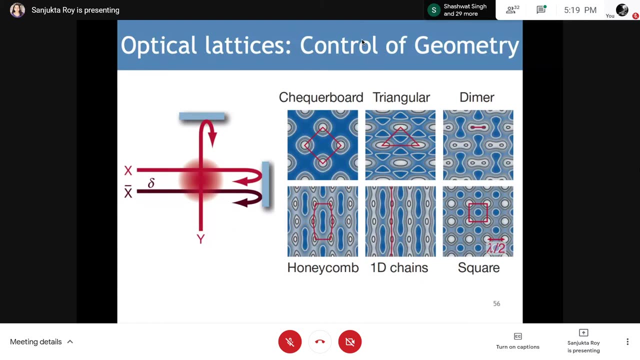 using the optical lattice, So you can go to 1D, 2D and 3D dimensions and explore a wide variety of physics by using Bose-Einstein condensate in what is called an optical lattice, So you can actually control the geometry of the beams. 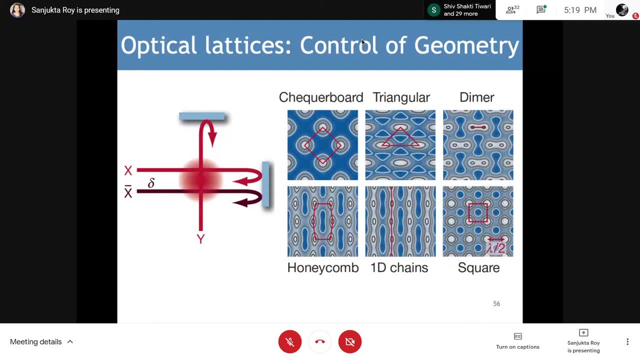 to realize a variety of optical lattice, like a checkerboard, triangular, dimer, honeycomb lattice, which are very important, And you can also control the geometry of the beam to realize graphene physics. So next I come to quantum simulation. 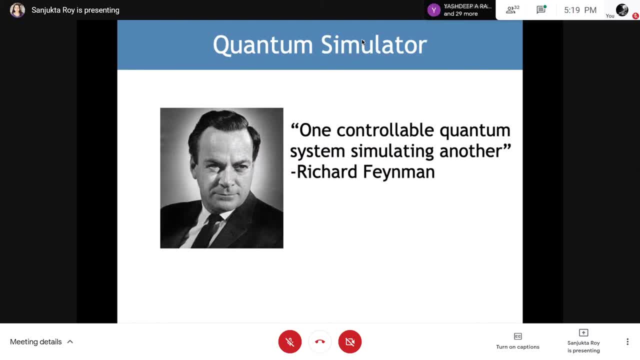 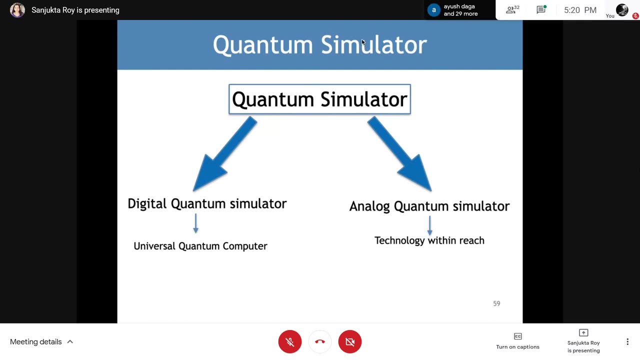 So what is a quantum simulator? So, according to the words of one of the greatest physicists, Richard Feynman, quantum simulator is one controllable quantum system simulating another quantum system. So you can have two kinds of quantum simulator. One is a digital quantum system. 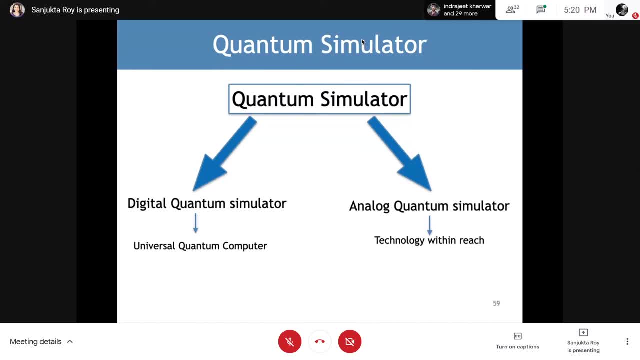 One is a digital quantum system. One is a digital quantum system, One is a digital quantum simulator, which is actually the universal quantum computer, which is yet to be completely realized. But we can have another kind of quantum simulator, which is the analog quantum simulator. 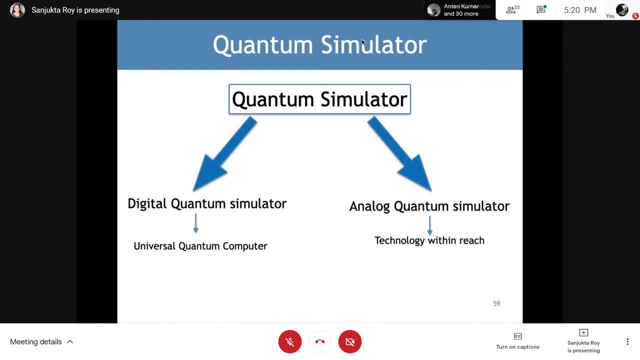 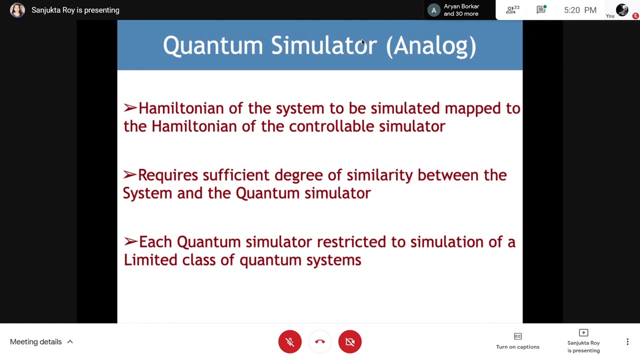 And we have the technology for analog quantum simulator completely within our reach, And that is what my main theme of the experiments which I'm going to describe now. Now, for the analog quantum simulator, we need a quantum system which has to be mapped to the Hamiltonian of the simulated quantum system. 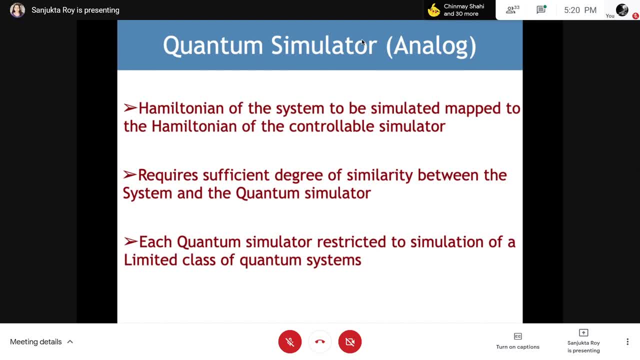 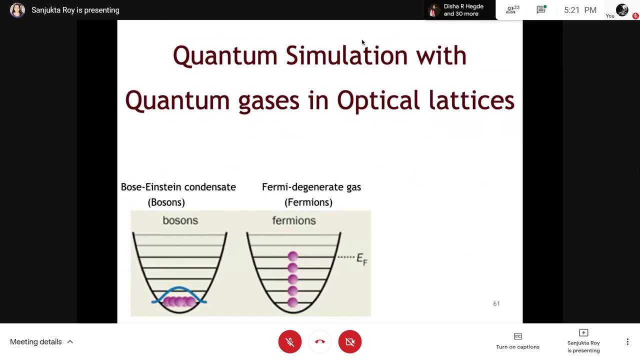 Now it should have a sufficient degree of similarity between the system which we are simulating and the quantum simulator. So we can use once and fermions to do the quantum simulation, or we can use as we are going to do in our experiment at RRI. 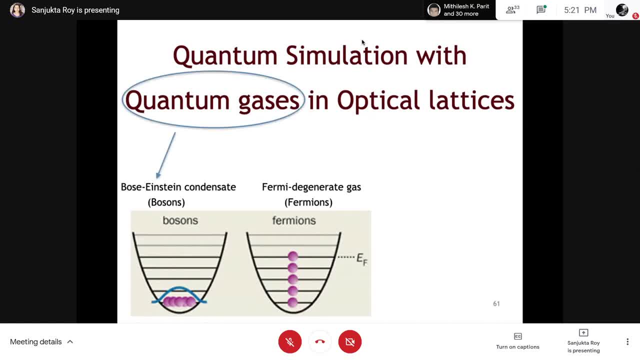 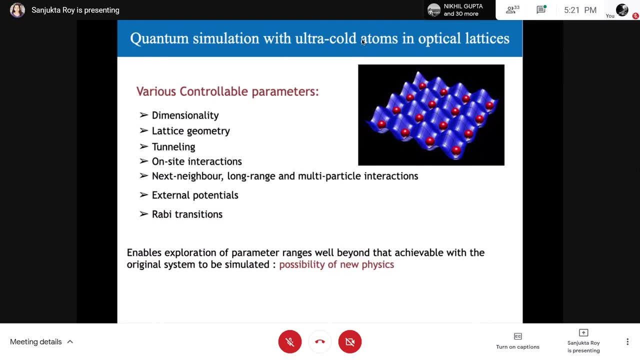 a mixture of boson and fermions. So why it's so much advantageous to do quantum simulation with ultra-cold quantum gases and optical lattice. As you may have realized, we have so many controllable parameters We can control the dimensionality. 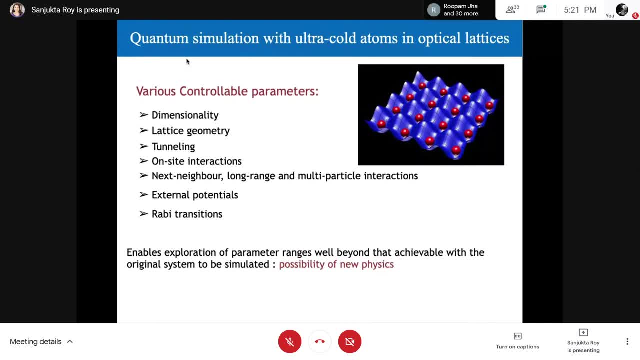 We can control the lattice geometry, We can control the tunneling between the lattice sites, We can control the interactions And we can control the external potentials. So we can actually control the system parameters in the same way as we do numerical simulation in a computer. but it's not. 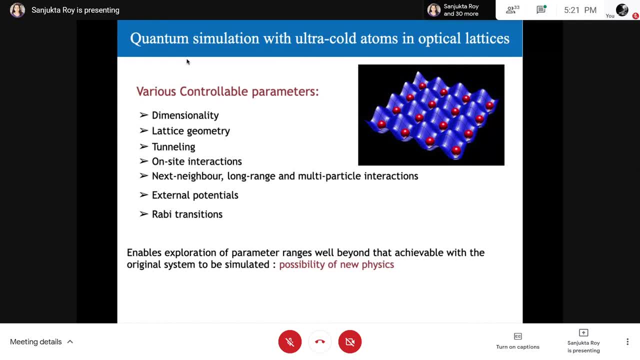 But it's actually done in a real system with atoms. So it also enables to reach parameter range which may be not even achieved in the real system. So you can have possibility to to explore new physics by doing those quantum simulation. so there are a lot of. 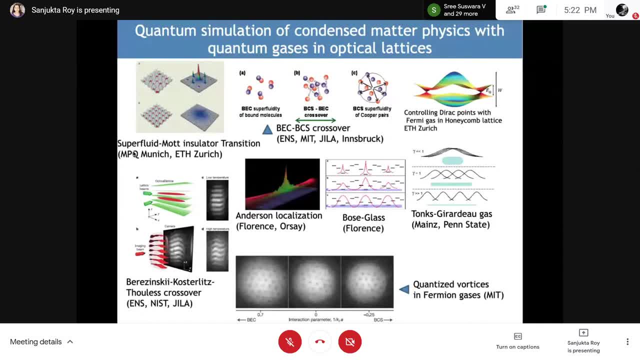 variety of quantum simulation which has been done with quantum gases and optical lattices. we have superfluid to mod insulator transition. we have something called a BC to BCS crossover, which has been done using fermionic atoms. we have, I mean, in in other groups. there have been simulation of graphene physics using. 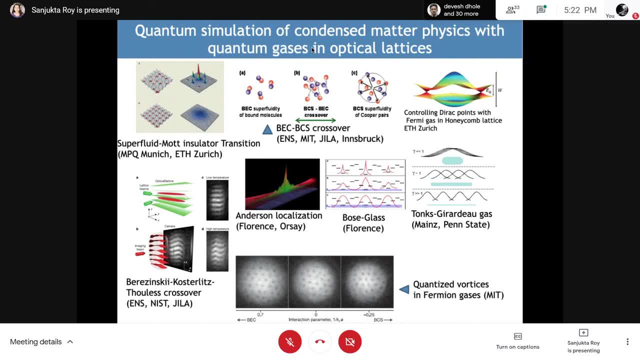 BC in honeycomb lattice. there have been. there have been also simulation of two-dimensional physics like BKT transition and of course there is Anderson localization, which I'll be talking about in a few slides, and also quantized vortices which I have shown a few sites ago. so there is a 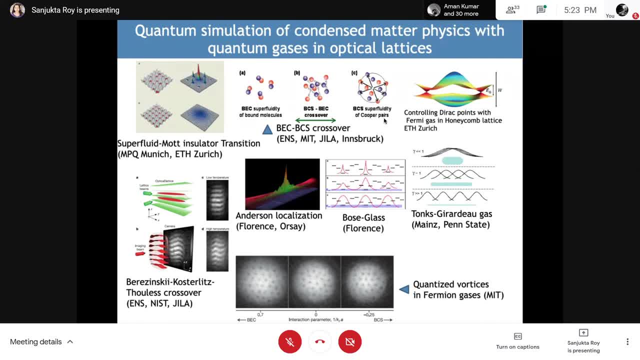 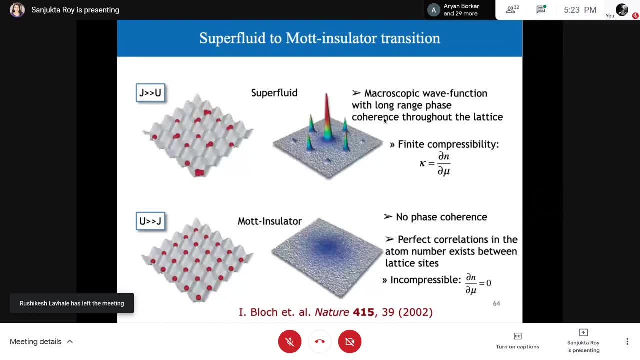 wide variety of physics which you can do using quantum gases in optical lattices. so one of the very important phenomena which was a and one of the first first results which act with quantum gases is superfluid to mod insulator transition, which was actually realized, realized in MPQ Munich, where the quantum gases in optical lattices 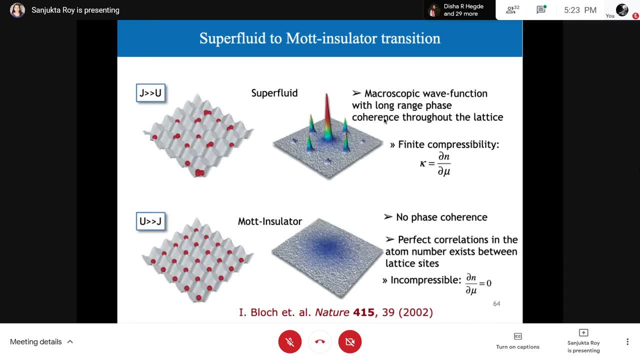 where, when you have the tunneling energy much, much higher than the interaction energy, the BC was like a superfluid in the optical lattice and when the interaction energy was dominating, what you bought insulator. so this is a pure condense matter phenomena which was realized in a very well controlled, clean 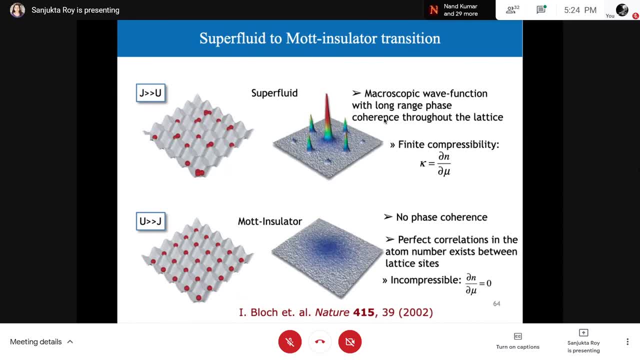 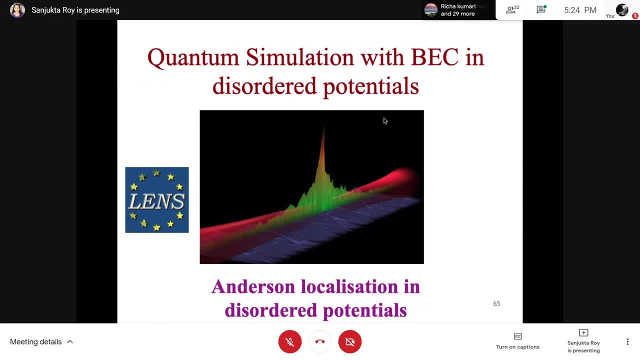 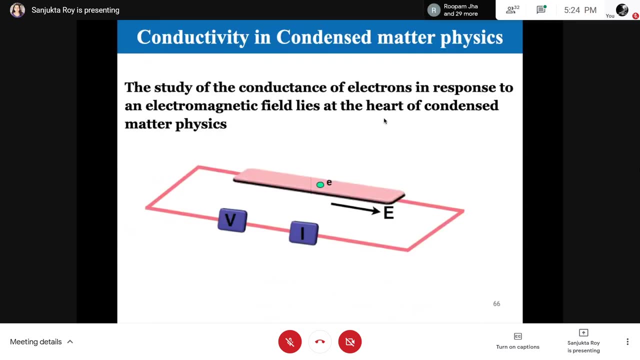 system in with a quantum gases in optical lattice. so next slide, please. I'll talk a little bit about quantum simulation with BC and disordered potential, which I had done during my postdoc in Florence. so, as we know that conductivity is is the main, one of the main areas of study in condense matter. 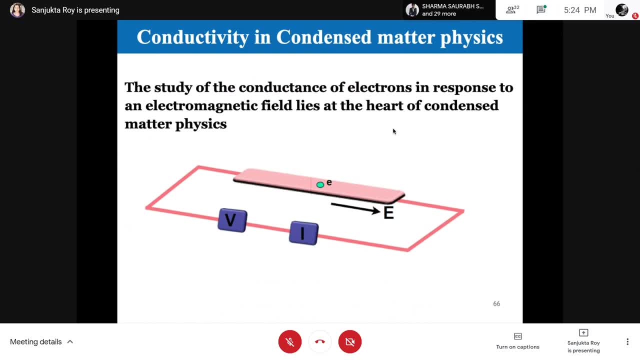 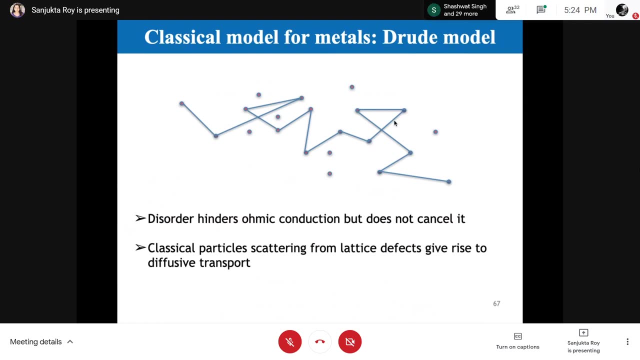 physics. so study of the conductance of electron in response to an external electromagnetic field is actually the heart at the heart of condense matter. physics. now for the classic. from the classical model for metals it was believed that disorder or randomness in in a solid-state lattice. it actually hinders. 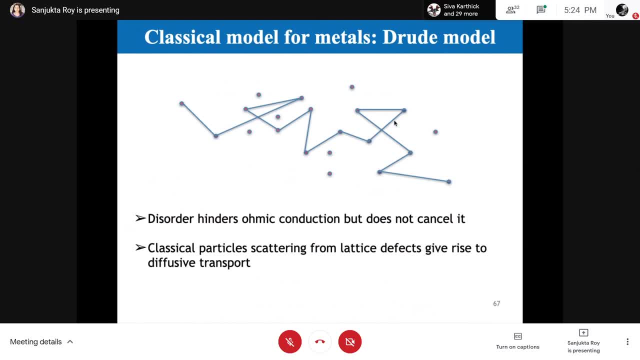 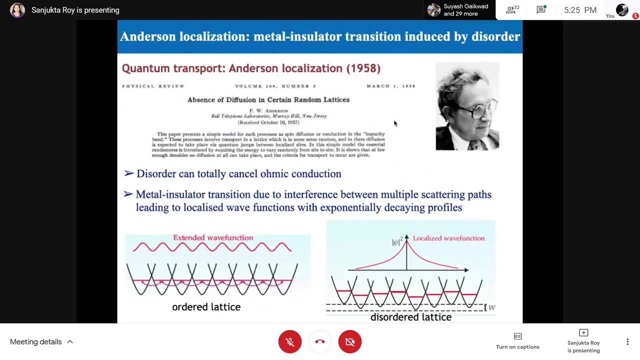 ohmic conduction, but it cannot cancel it, and so classical particles, which were scattered, scattered on the lattice, defects were actually giving rise to diffusive transport. but there was a paradigm shifting paper by Anderson who, in 1958, said that disorder or randomness in in in a solid state lattice can. 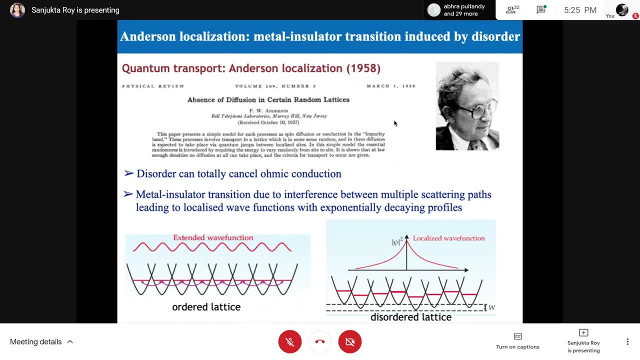 completely cancel the conduction. so he predicted a metal insulator transition due to interference of multiple scattering parts which led to localized wave functions with the characteristic exponentially decaying profile. so if you have, or that lattice which is on the left, you have an extended wave function, but when you have a disordered lattice site due, 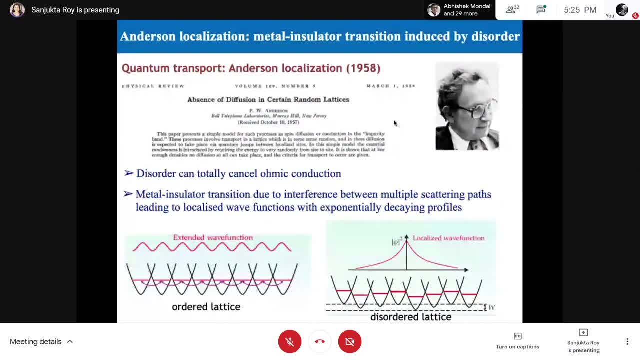 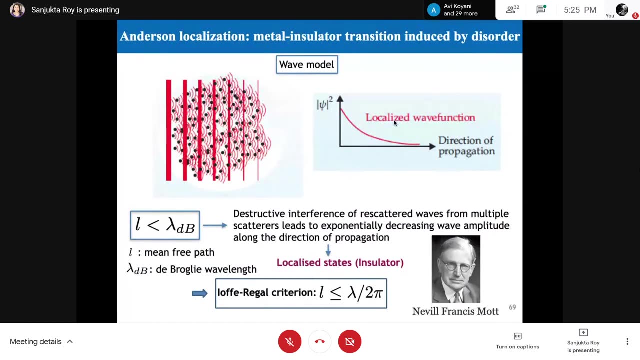 destructive interference of the of the scattered waves, scattered matter waves, you get a localized wave function with exponentially decaying profile. so, uh, one condition which is has to be satisfied to have the anderson localization, which is called a i of regal criteria, which is that the mean free. 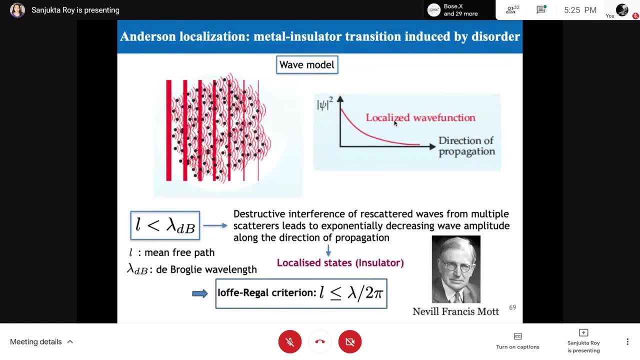 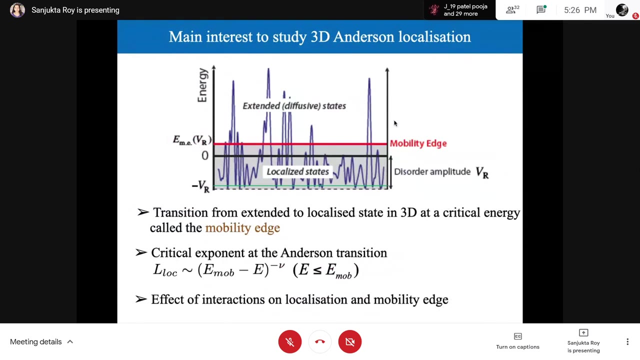 path should be less than the d broccoli wavelength. so the destructive interference of the re-scattered matter waves from the multiple scattered in a disordered lattice actually leads to exponentially decreasing wave amplitude, uh, which actually leads to anderson localization. so, uh, what i did in florence is a 3d anderson localization. so, um, the 3d anderson localization is actually. 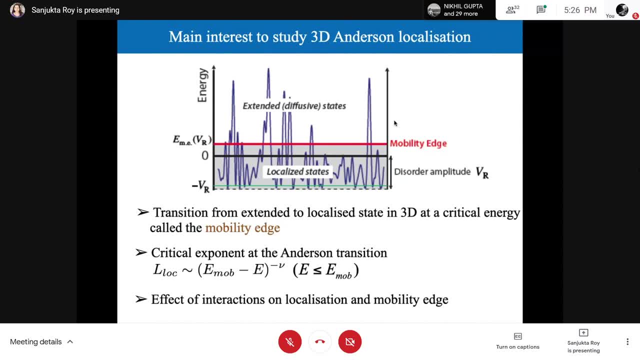 characterized by a critical energy called the mobility edge, which actually marks the transition from a diffusive state to a localized state when you decrease, when you increase the amount of uh, the amplitude of the disordered potential. so this critical energy was not uh precisely measured before, but we needed it very uh, i mean this mobility edge. precise measurement of mobility edge was very. 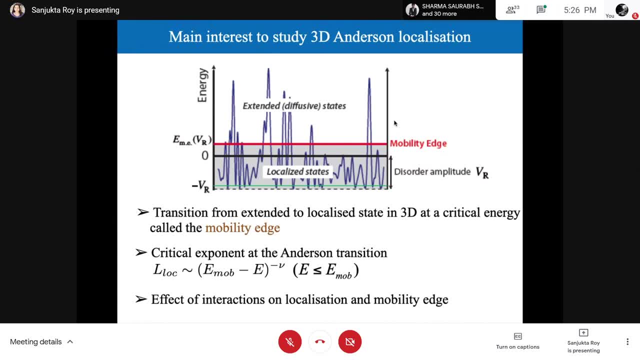 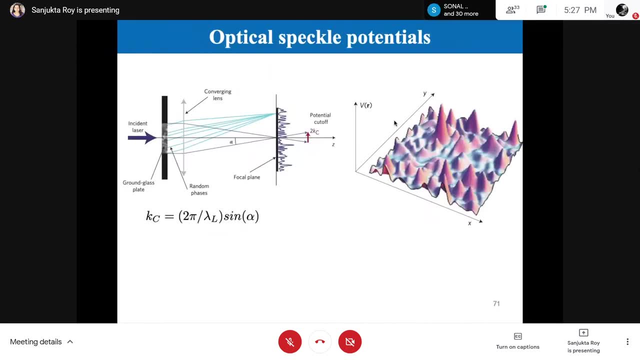 very much needed to actually uh resolve a lot of, uh you know, open problems in in disordered physics. so we actually uh uh loaded the bc, or the quantum gases, in a disordered optical potential. so we- how do we make that disordered potential is actually uh passing the laser beam through a 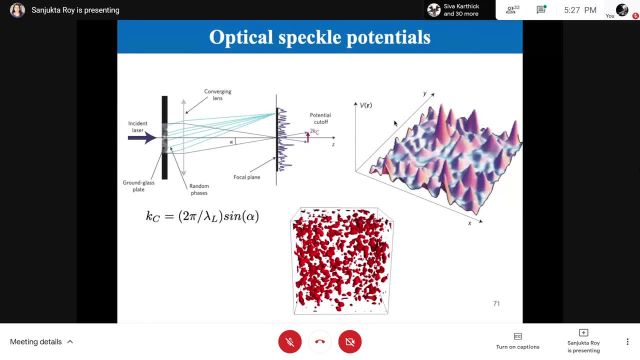 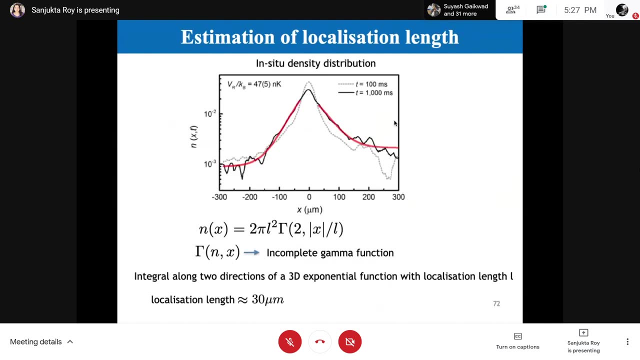 diffusive glass plate and actually forming a random potential at the place where the atoms were trapped. so atoms were actually um loaded in a disordered optical potential and hence by controlling the appropriate parameters we could realize a 3d anderson local localization with the characteristic exponential decaying profiles. 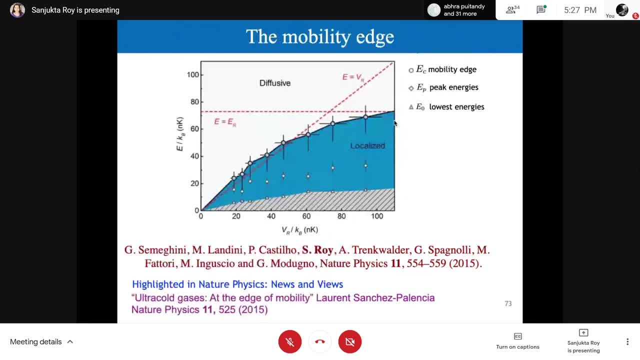 as you can see in the figure. so here we could have a very precise measurement of the mobility edge which actually marks the phase transition to the anderson localized phase. so this is one of the uh very important quantum simulation of uh simulation of disordered condense matter physics, which 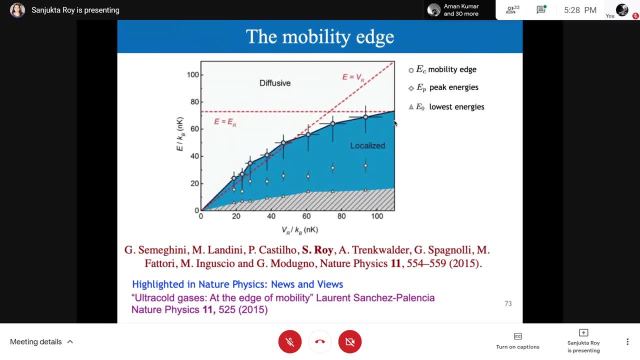 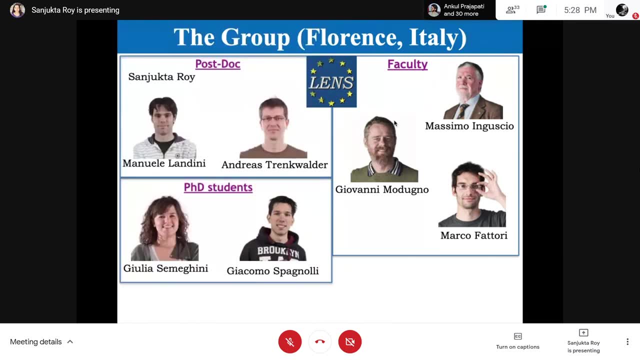 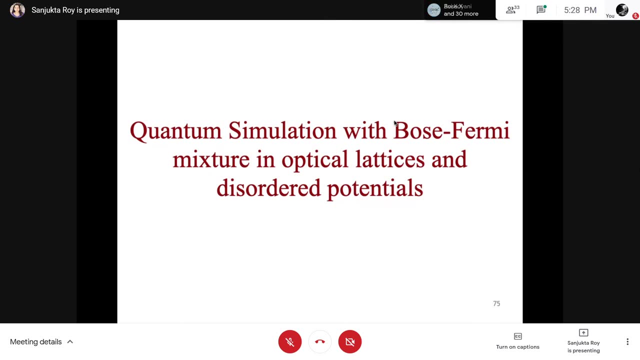 we have done using ultra cold atoms in uh, disordered optical potentials. so this is, this was our group in florence, italy, which who have uh together done this work. now here i uh. it's the last part of my talk where i actually talk about quantum simulation with Bose-Fermi mixture in optical lattices, which, for my, my meta research and visualization, which i have really been interested in doing for many years in chiaroscuro. 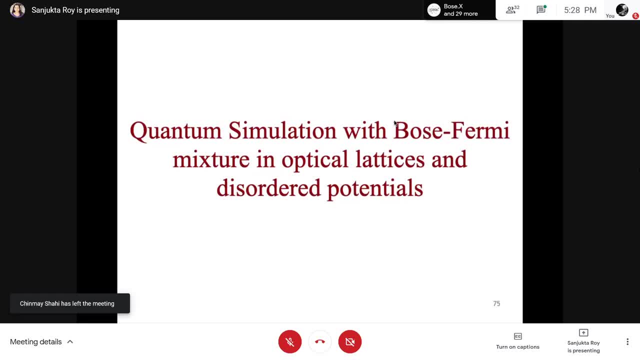 so this is, uh, a really interesting project and they just simply Photoshop and an origination of the moment, light, current activity. they had some very interesting projects again. they developed an organization called plasma which позвол guide these kinds of simultaneousorthic meaning of the throughout quantum, arbitrary Fer explosive mass. 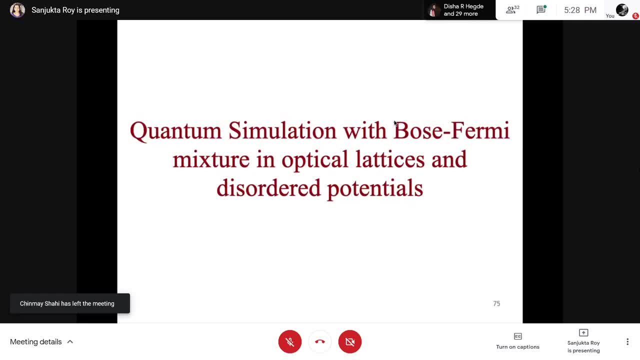 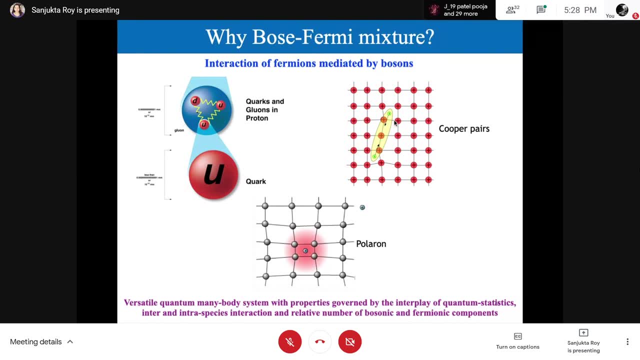 analysis which we are pursuing presently at Raman Research Institute. So why Bose Fermi mixture is important Because it's everywhere in nature. you have interaction of fermions mediated by bosons. For example, in standard model you have the interaction between the fermionic particles. 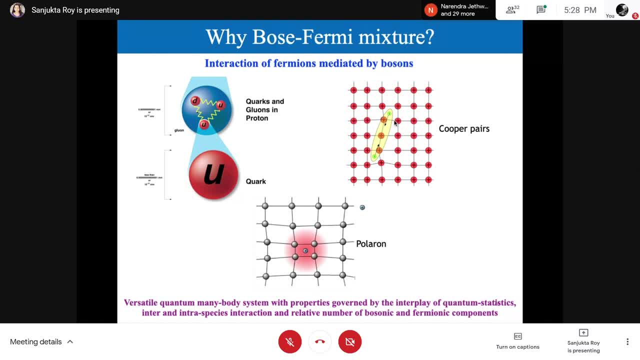 They are mediated by gauge bosons. You have the quarks, which are fermions Between them. the interaction is mediated by gluons, which are bosons. Also, you have the electrons dressed by the lattice vibrations of the ions which forms. 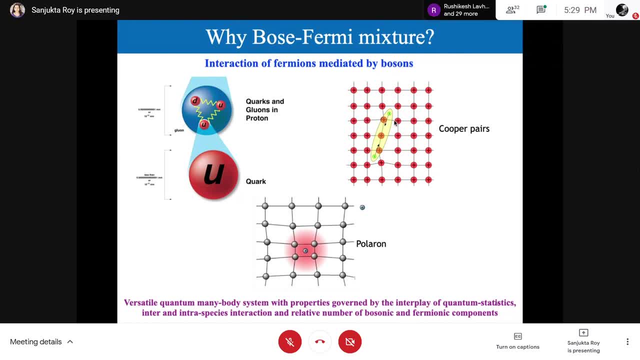 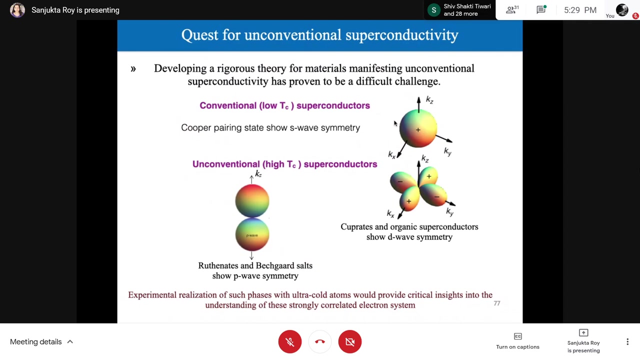 polarons. And also we have the interaction between the electrons in a Cooper pair is mediated by phonons. So you see that how everywhere in nature you have bosons mediating the interaction between the fermionic particles. So we have a few ideas where we would like to quantum, simulate condensed matter physics. 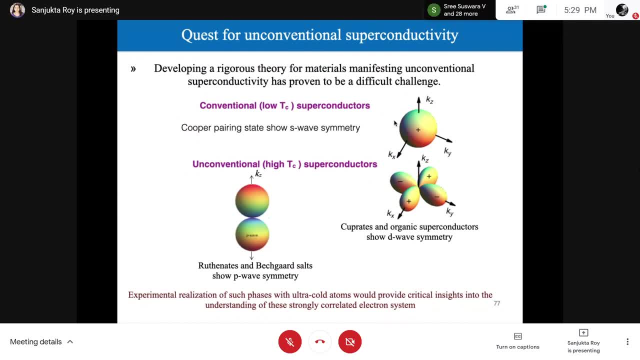 where there are open problems, using Bose Fermi mixture in optical lattices, For example. we all know that the rigorous theory for unconventional superconductivity or high temperature superconductivity is still an open problem, But here we can actually use Bose Fermi mixture in a 2D optical lattice to simulate unconventional 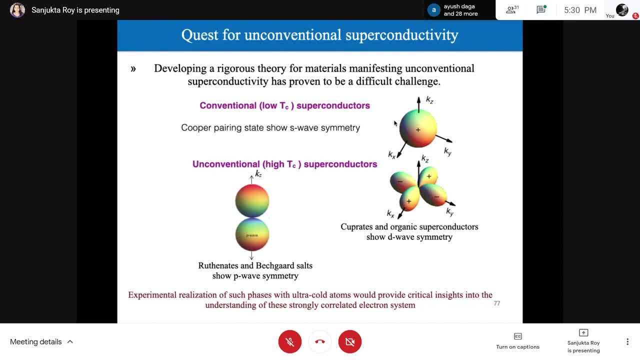 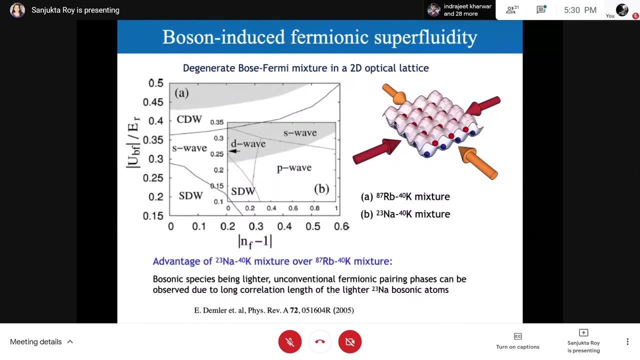 super fluidity or high temperature superconductivity, and explore the parameters which can give us understanding. So it has been predicted that if we have Bose Fermi mixture or a mixture of sodium and potassium, which is our experiment at RRI at present, if we have the potassium as the fermionic, 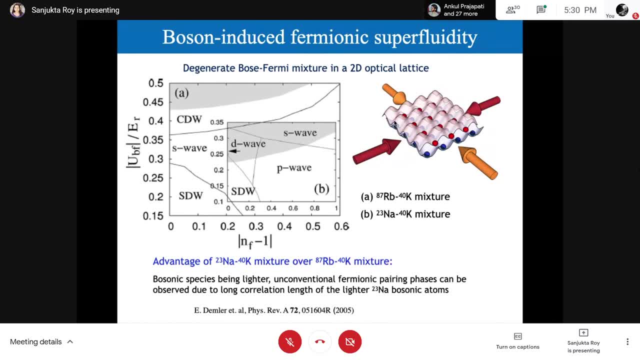 species and sodium as the bosonic species. the sodium being the bosonic species, can actually mediate the interaction between the fermions and actually can simulate the physics of the physics of unconventional super or high temperature superconductors and which is actually given by the signatures, like charge density wave or D-wave or P-wave, super fluidity, which are 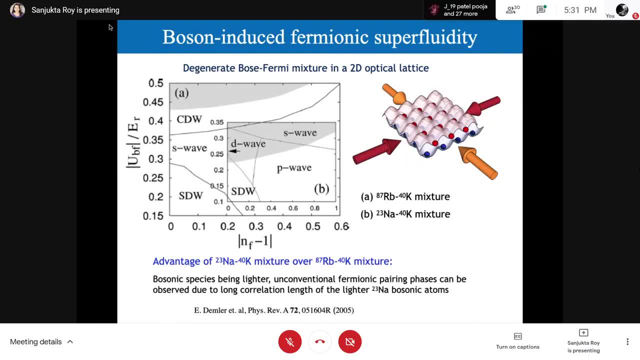 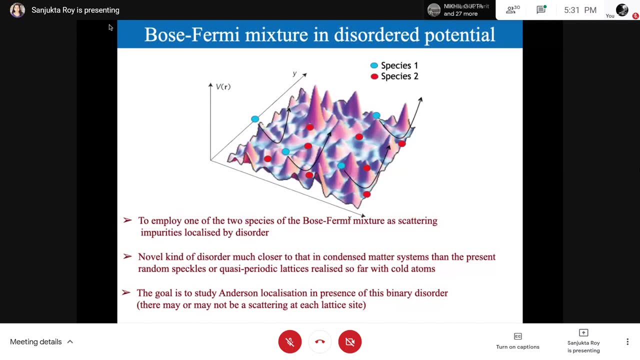 the signatures of high temperature superconductors. Also, we can have Bose Fermi mixture in disordered potential, where we can have one species actually trapped in the disordered potential and that giving rise to scattering of the other species. So this is actually will be enough. you know, Anderson, localization where one atomic species 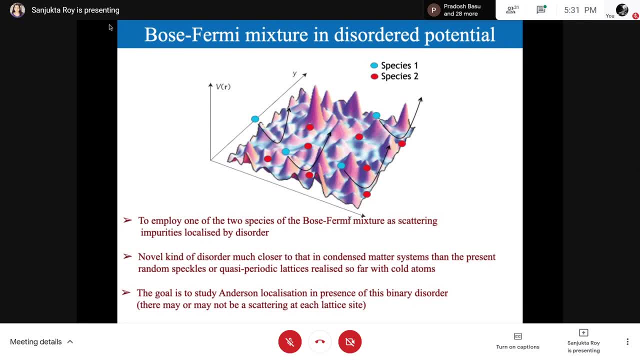 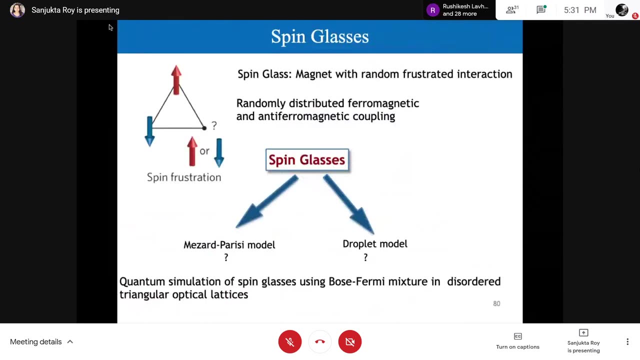 is actually causing a disordered potential for the other atomic species. So these kind of open problems have not yet been addressed in condensate matter physics, as well as in ultra cold atom physics Also, we have something interesting in mind to explore with Bose Fermi mixture. 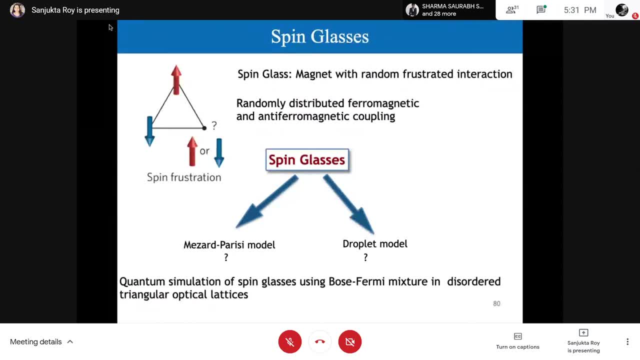 So this is an example. This picture is something called a spin glass where we have- we have a spin in disordered potential with random interaction. So if you have spins in a triangle as well as in a disordered potential, you have something called a random coupling and a frustration. 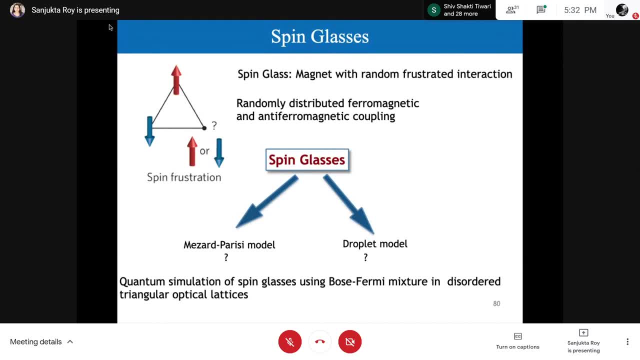 So if you have in a triangular lattice, so if you have spins, if you want to have opposite sides of the triangular lattice, so it creates some kind of frustration because it has. so the spin doesn't know which way to point and this leads to frustration. 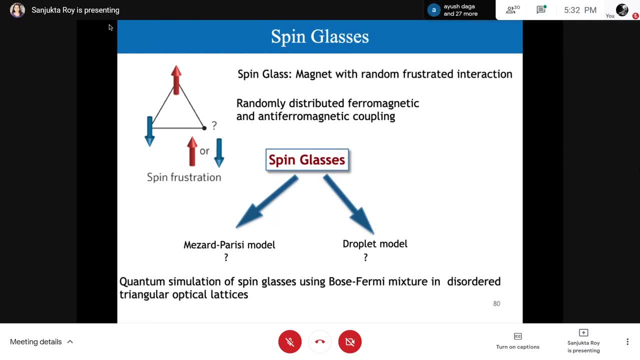 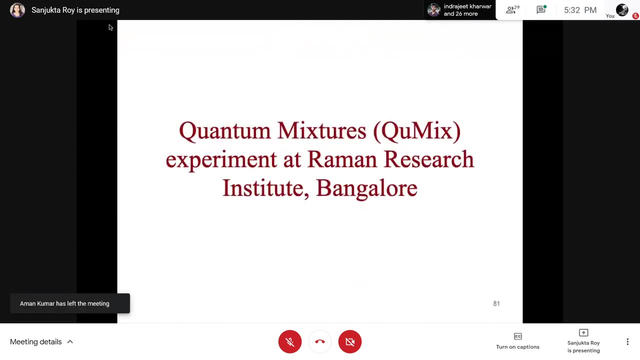 And this is actually the basis of spin glasses. So we were, we are going to use Bose Fermi mixture in disordered triangular optical lattice to address this open problem of spin glasses. So now I show the quantum mixture experiment at Raman Research Institute. 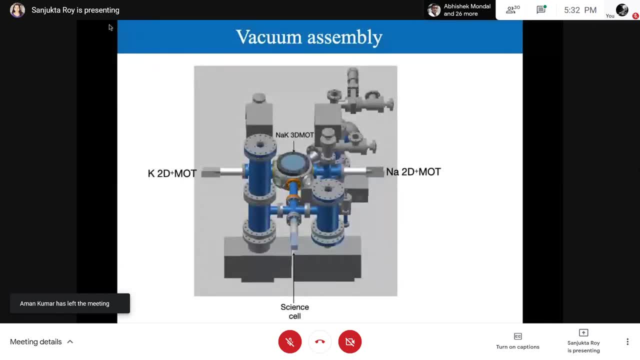 So here we are actually building up an experiment of sodium and potassium, where potassium will be the fermionic species and sodium will be the bosonic species. So we have an experiment where we have a two, two, two dimensional 2D plus magneto optical. 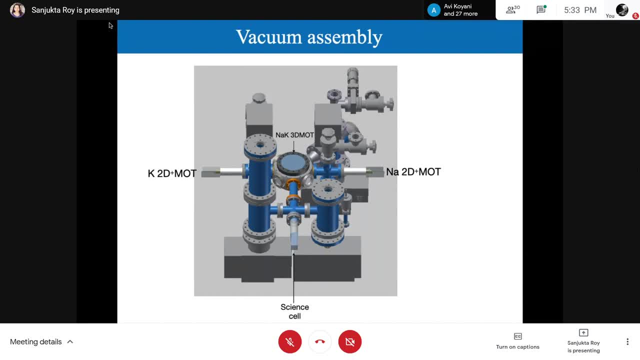 trap for sodium and potassium which will actually load a single 3D board which will give a mixture of sodium and potassium in the magneto optical trap. So this is an example, And then we will have a magnetic transport which will load the mixture of cold atoms.